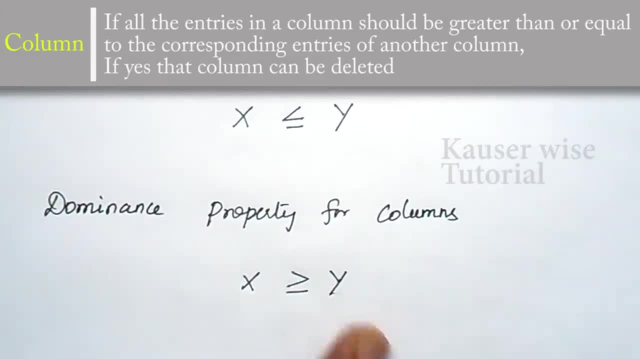 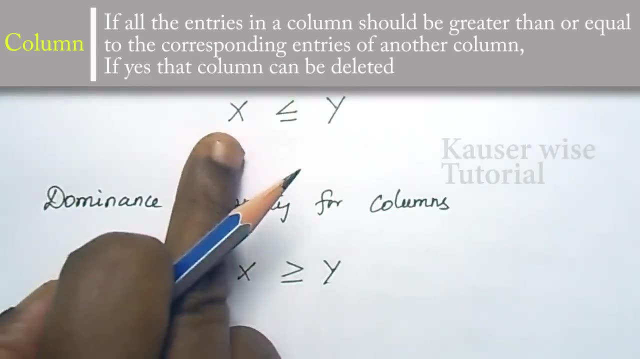 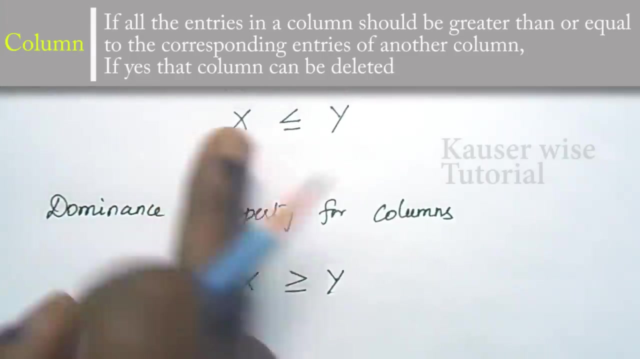 column x is dominated by column y. So therefore, delete column x from the pair of matrix. When you take row, delete the least value. When you take the column, delete the highest value because player a is a gainer and player b is a loser. So this is the general dominance property. 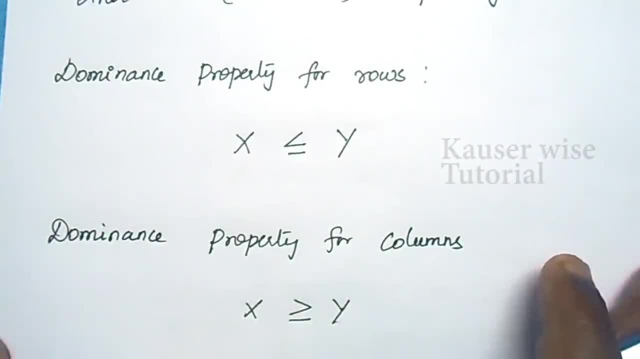 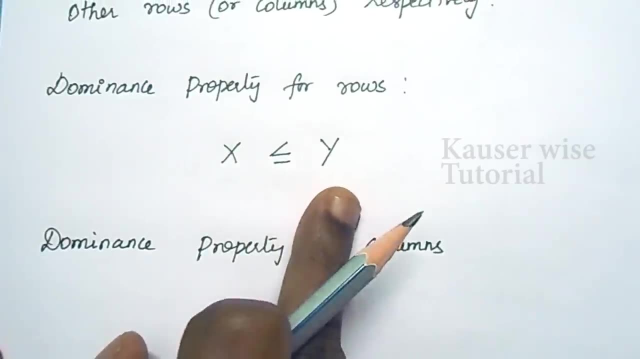 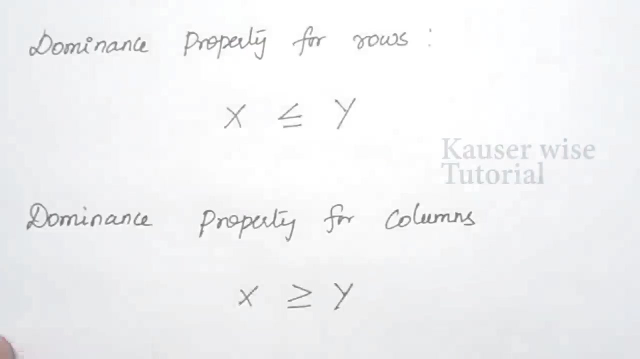 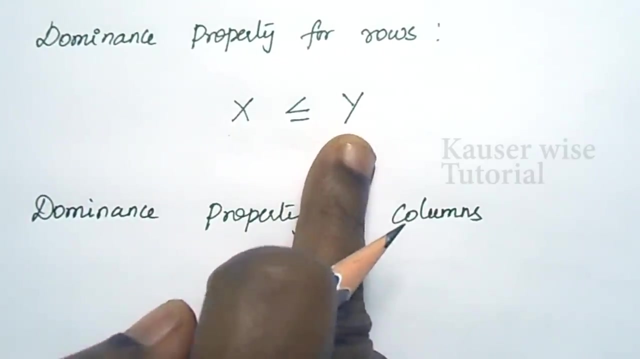 In some cases, we can compare one particular row or one particular column along with the average of two or more rows, or two or more columns, in order to reduce the pair of matrix. Again, I repeat, you can compare one particular row with the average of two or more rows in order to eliminate. 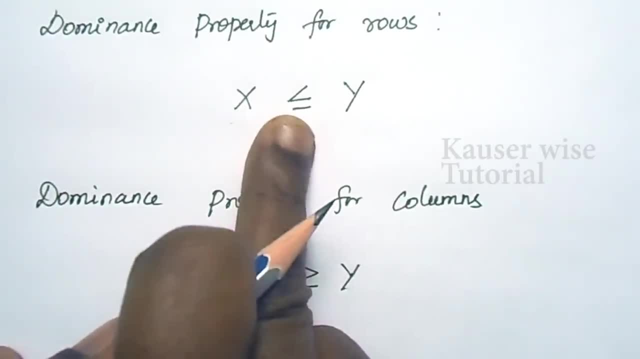 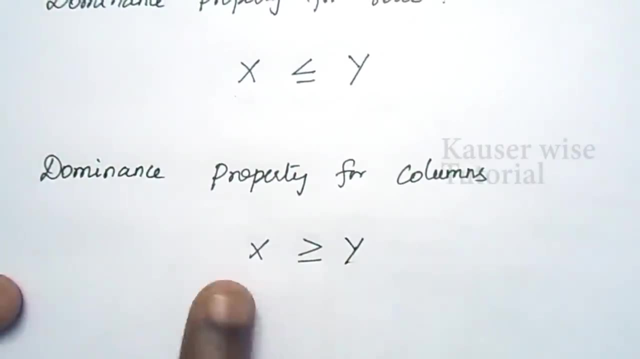 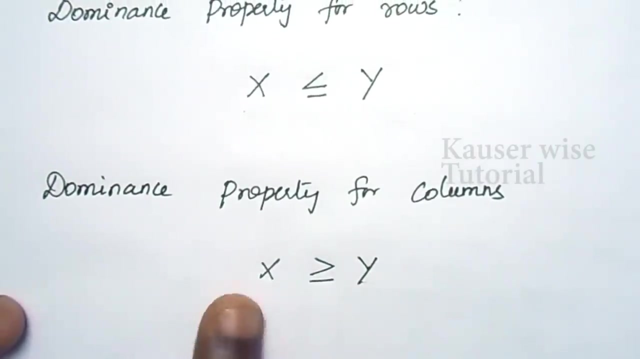 to check whether the particular row is lesser than or equal to corresponding elements of another row. The same thing is applicable for column. also. You can compare one particular column with the average of two or more columns to check whether the particular column is greater than or equal to. 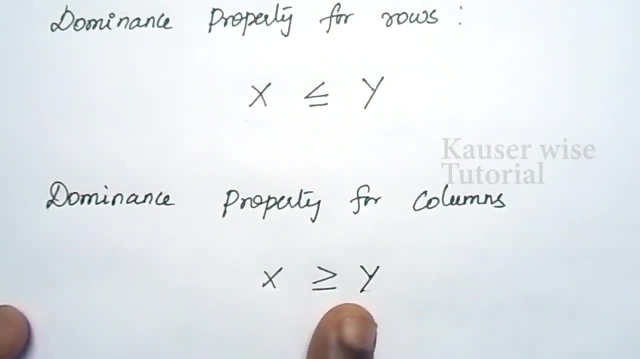 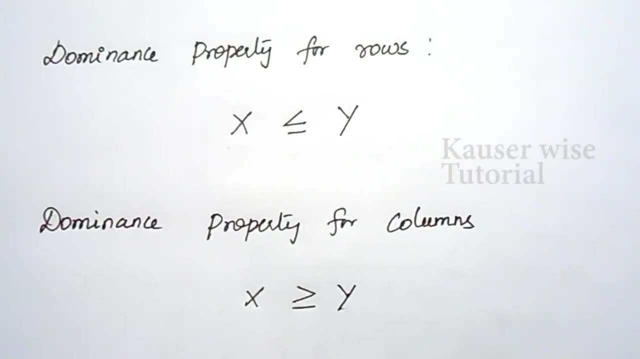 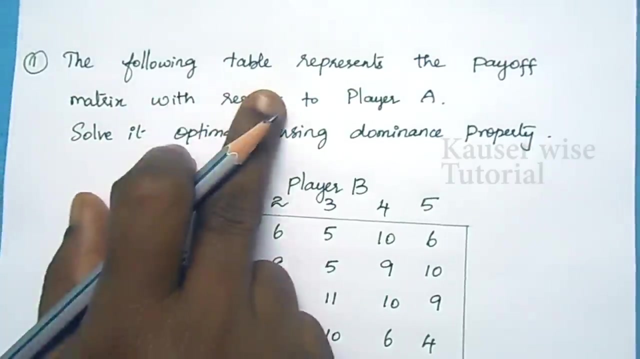 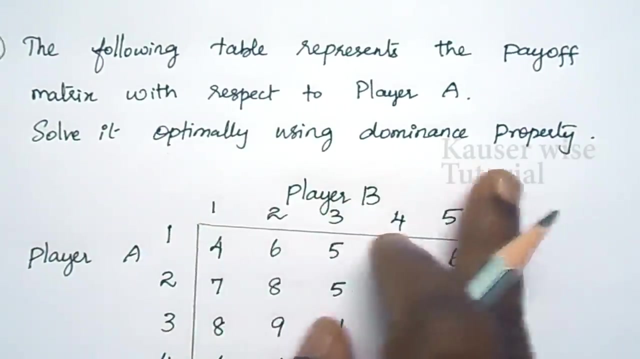 average of two or more columns in order to reduce the pair of matrix. We will see this average method along with the problem in detail. The next problem for dominance property with pure strategy. Look at the problem. The following table: represent the pair of matrix with respect to player a. Solve it optimally using dominance. 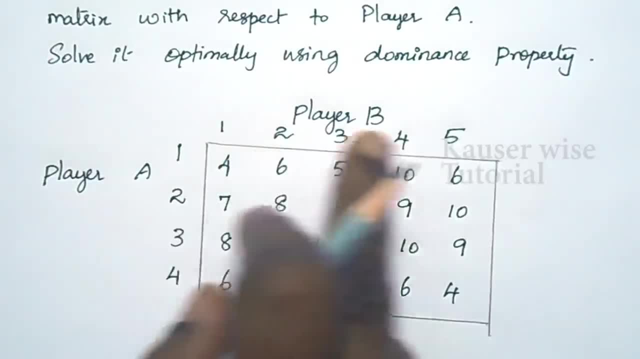 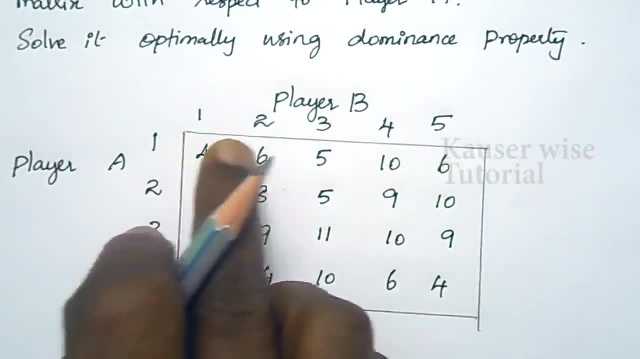 property. Here two players are there, player a and player b, and player a has four strategies: 1, 2, 3, 4, and player b 5 strategies are there: 1, 2, 3, 4, 5, and this is the outcome: pair of matrix. So now the 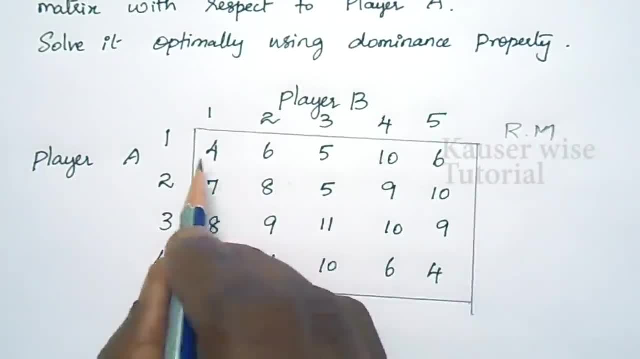 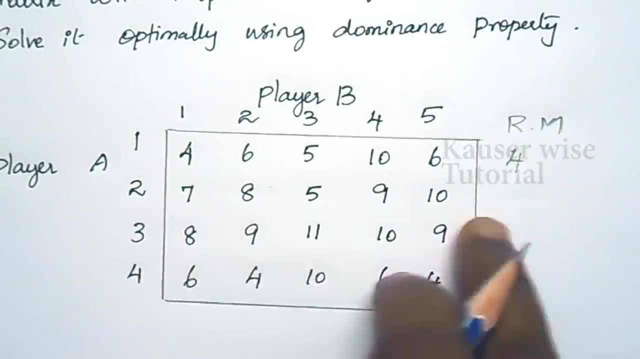 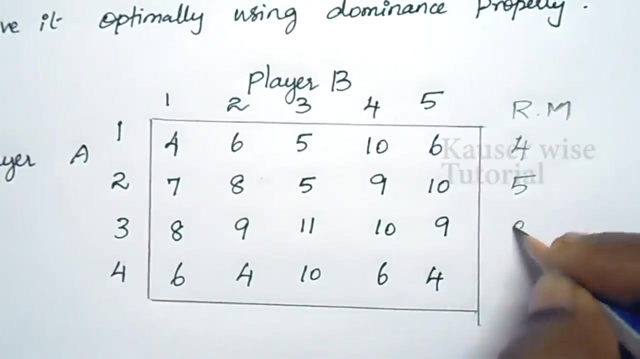 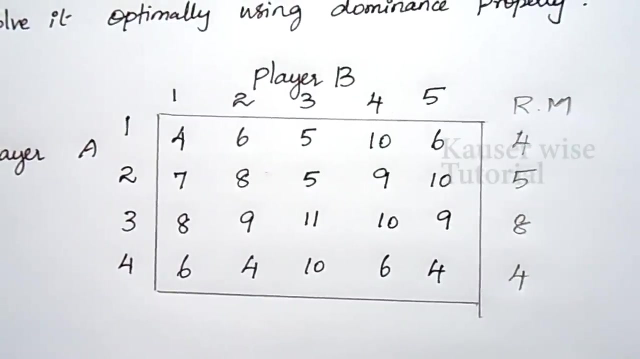 problem is solved. Find out the row minimum. Look at the first row. which one is minimum value? 4 is the minimum value, So write 4 here. Look at the second row: the least value is 5.. Third row: least value is 8.. Fourth row: least value is 4.. In the same way, find out the column maximum. Look at the. 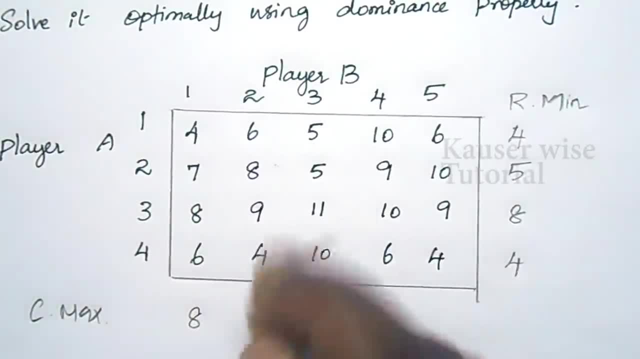 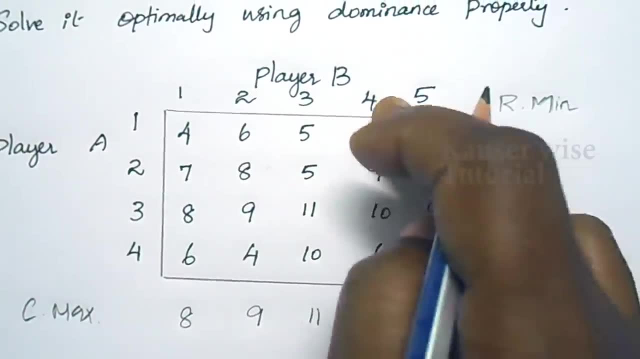 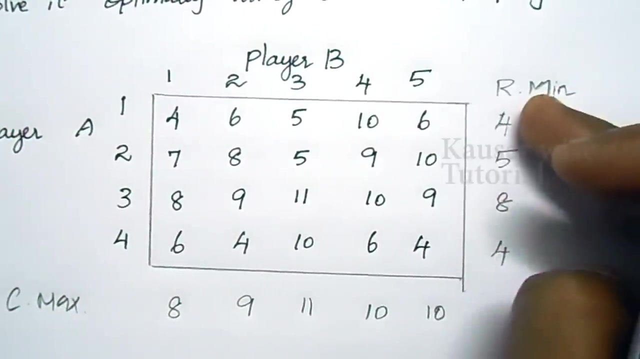 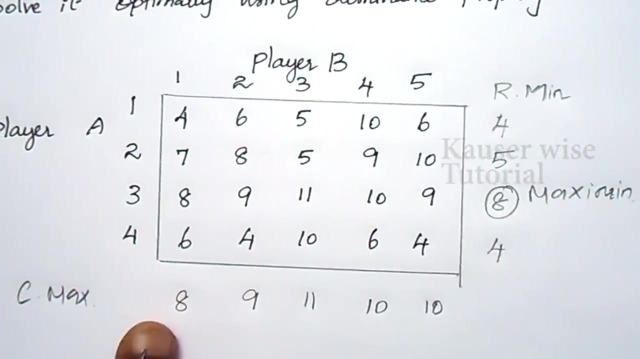 first column, maximum value is 8.. In the second column, maximum value is 8.. In the second column, 9 is the maximum value. The third column: 11.. The fourth column: 10.. The fifth column, again 10.. Now, among the row minimum, which one is maximum value? 8 is the maximum value. In the same way, find out. 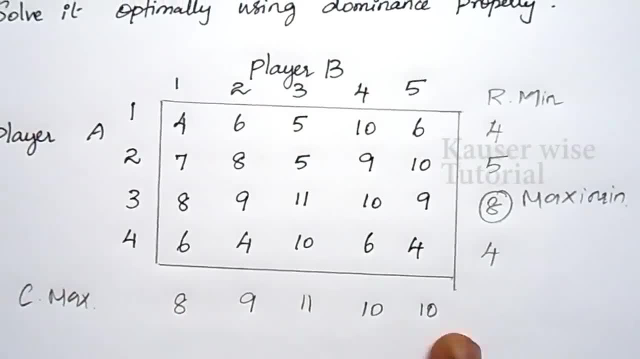 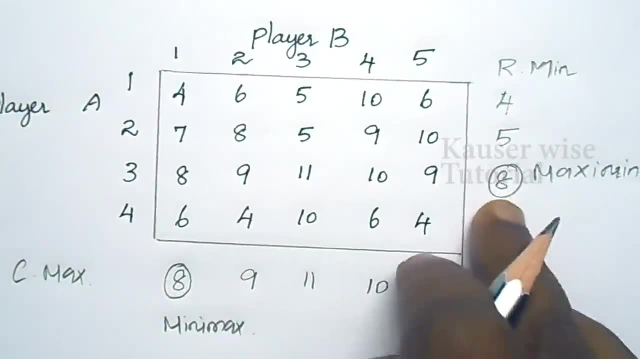 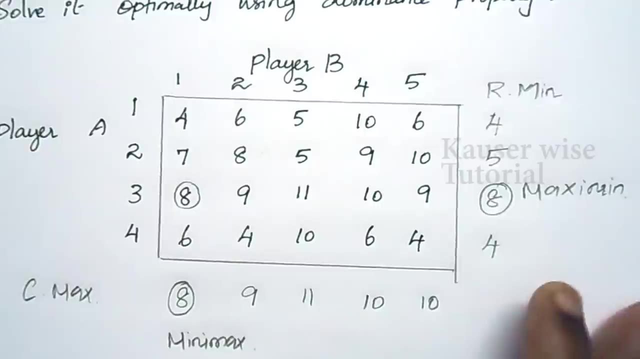 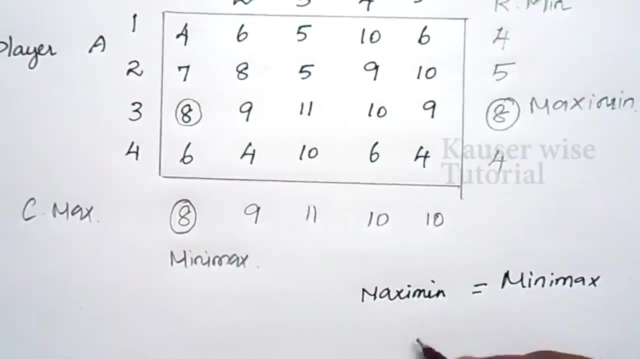 the minimax value. So among the maximum value, which one is minimum? 8 is the minimum value. That is the maximum value. Now the maximum value is equal to minimax value. No, So the value of game is 8.. Okay, See, this game has saddle point. The maximum value is equal to minimax value, So maximum value. 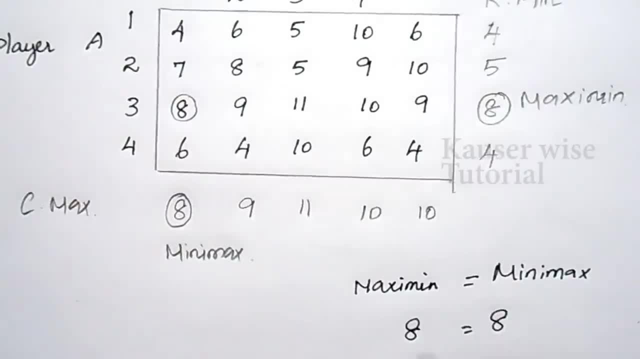 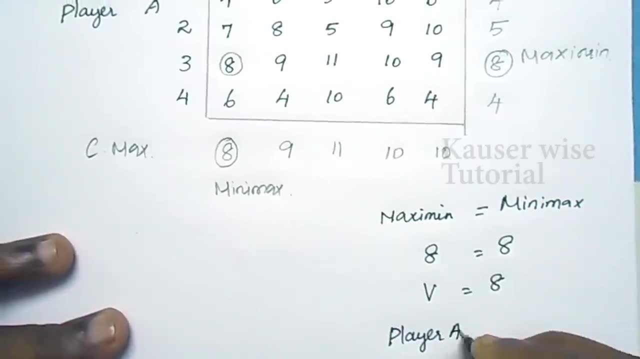 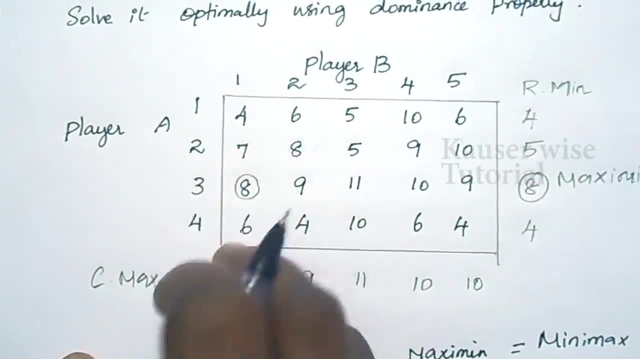 is 8- is equal to minimax value, also 8.. So the value of the game is 8.. So let me explain the probability of player a and b. Player a- the probability is player a- need to select the third strategy. Okay, So the remaining strategies are 0.. First strategy is 0.. Second, also 0.. He is going. 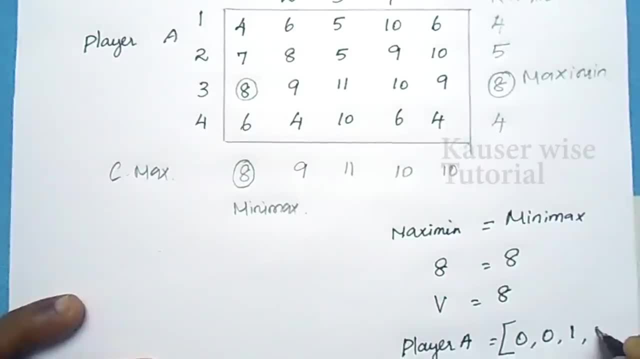 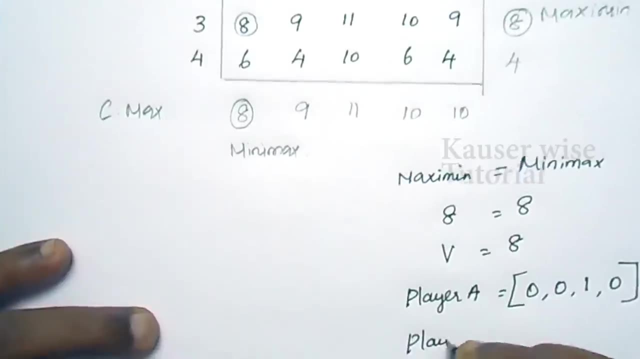 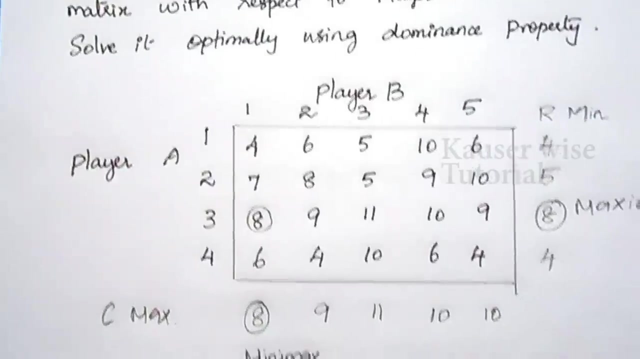 to select only one strategy, that is, third strategy and fourth strategy. also, probability is 0.. Okay, These are the probabilities of player a. In the same way, probabilities of player b is player b need to select the first strategy. Okay, So probability of player b is 1 comma 0 0, 0. 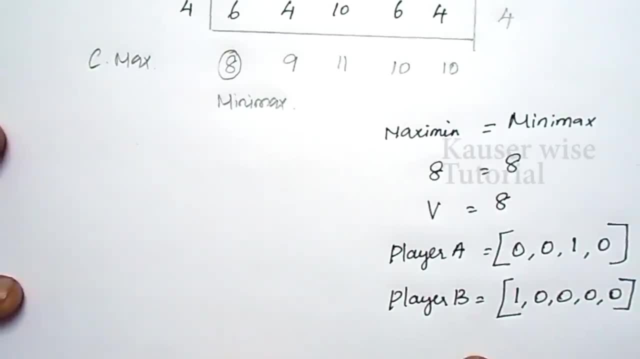 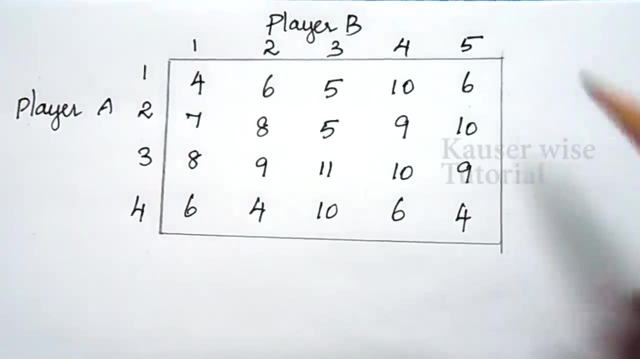 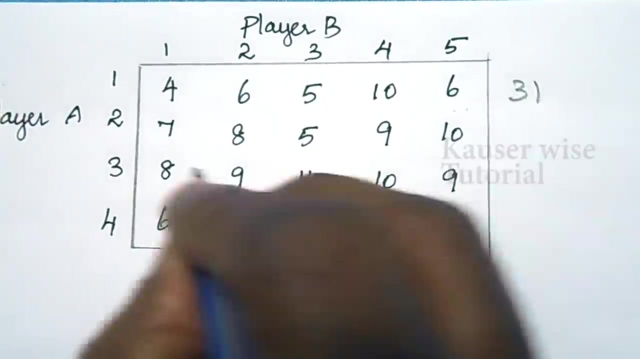 Now we are going to see the same result by using dominance property. Okay, Now let me solve the problem by using dominance property. Okay, The first step is we need to take the total of each and every row. Okay, The first row total is 31.. Second row: total 39.. Third row: total 47 and fourth: 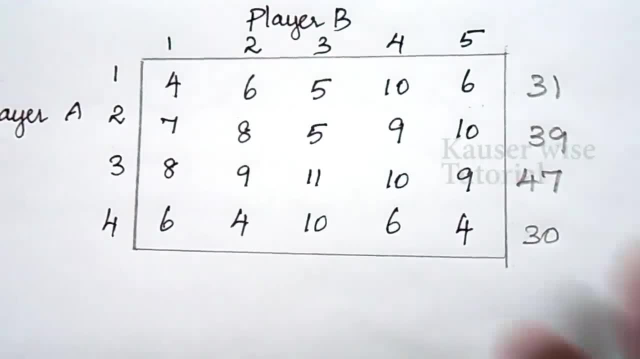 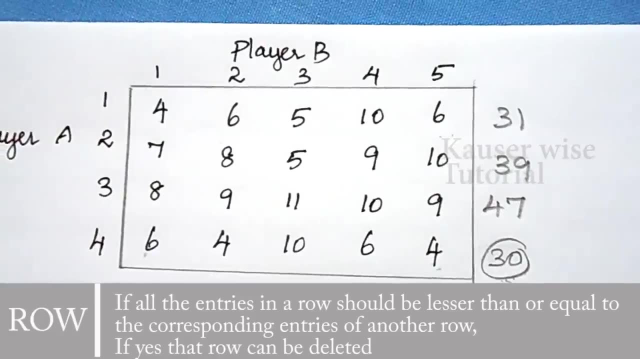 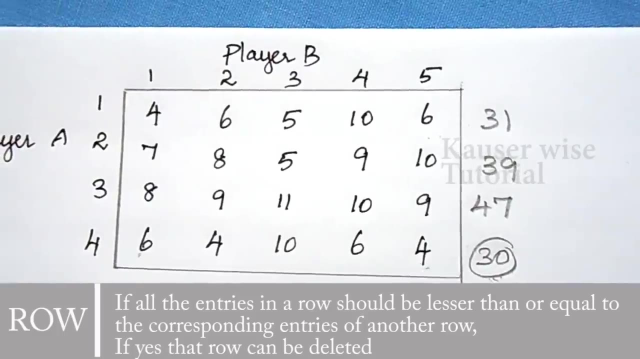 row total 30.. Now we need to select the least one, Okay. So what is the dominance property rule for row? Okay, If each and every row is lesser than or equal to any other row, then this particular row is dominated by other rows. So there you have to. 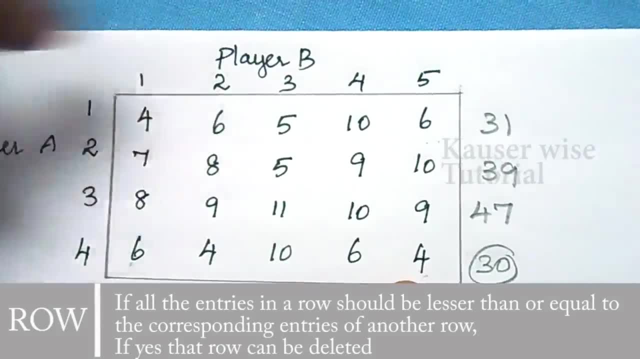 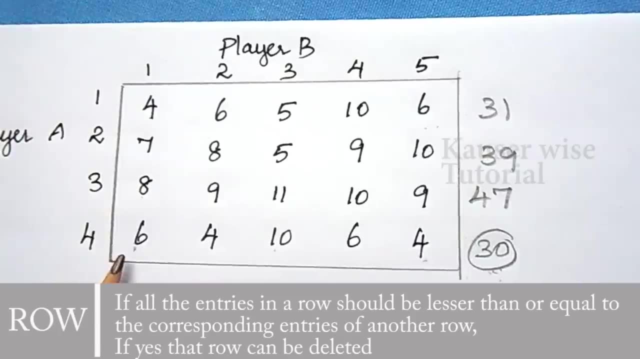 delete this particular row. So I am going to start from the first row. Okay, Look at the first row values and compare these values with the least value to check whether is there any continuous dominance or not. Okay, Look at the first value. So I am going to take the first row and compare. 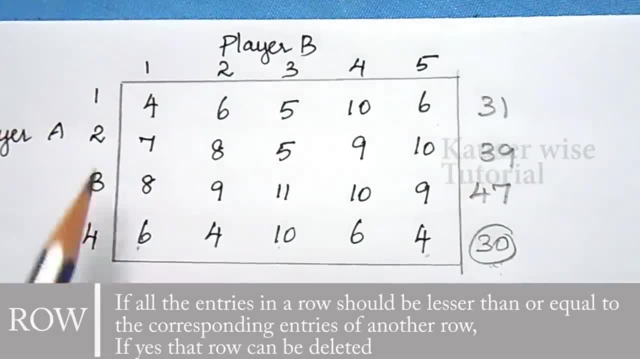 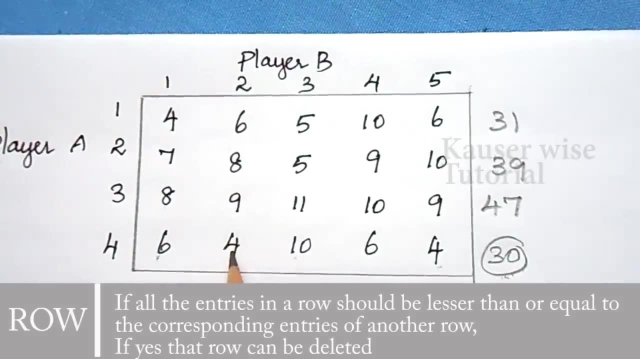 these values with the least value. So the first row is greater than or equal to any other row. Four, six is greater. So no domination. Go to the second row. Seven is greater than six, So six is a lesser value. Four is a lesser value. Ten is higher. Okay, So no domination. Go to the next. 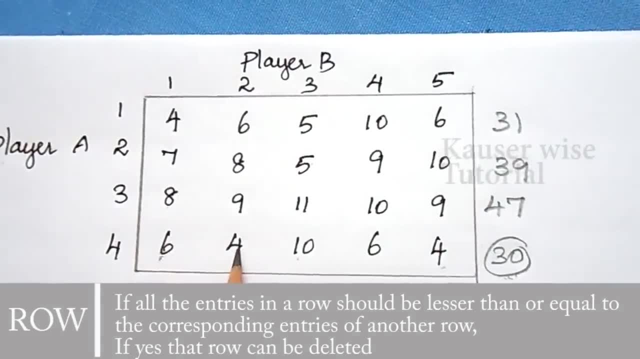 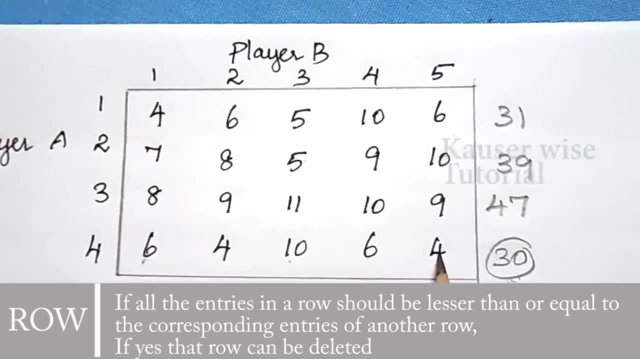 option Eight. Six is lesser than eight, Four is lesser than nine, Ten is lesser than eleven, Six is lesser than ten. Again, four is lesser than nine. So this particular row is dominated by this row. So delete this particular row. 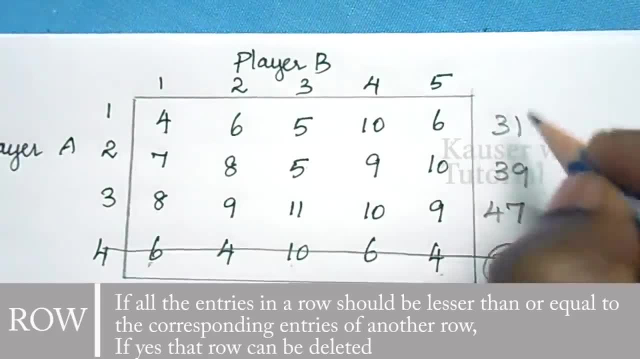 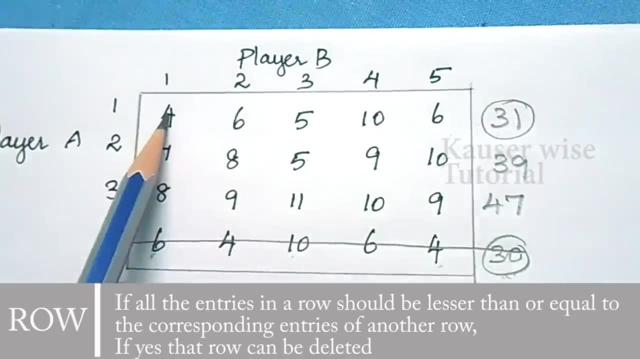 Now next one. So next least value is 31.. Now I am going to select this row and I am going to compare these elements with other rows. So 4.. 4 is lesser than 7.. 6 lesser than 8.. 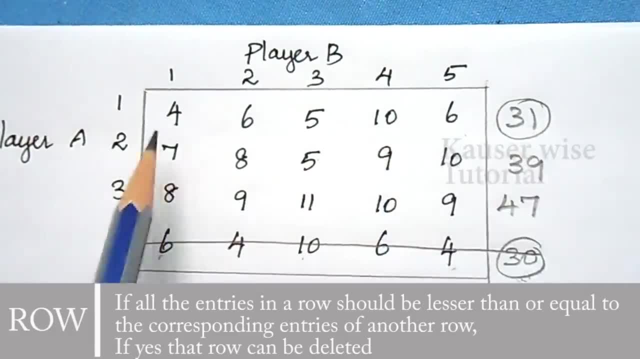 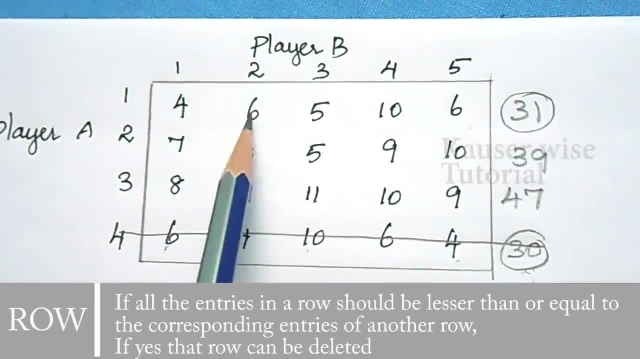 5 is equal, 10 is greater, So no domination. Go to the next option. 8 is there, So in this row the first value is 8.. So 4 is lesser than 8.. 6 lesser than 9.. 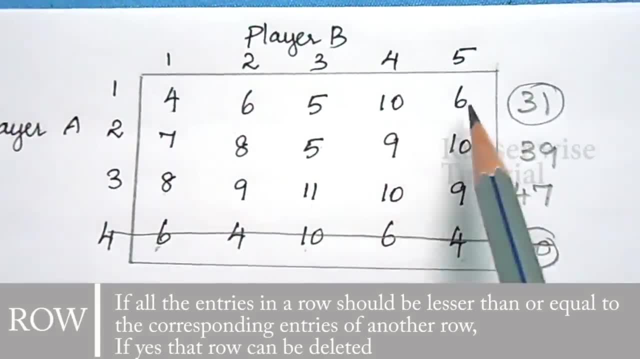 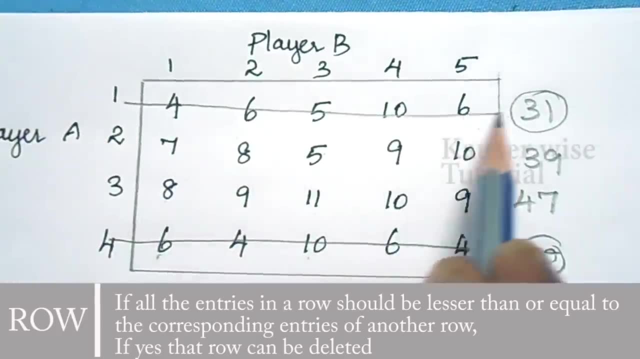 5 is lesser than 11.. 10 is equal, 6 is lesser than 9.. So this particular row is dominated by this row. So delete this particular row, Okay. Still, we have 2 rows, Okay. 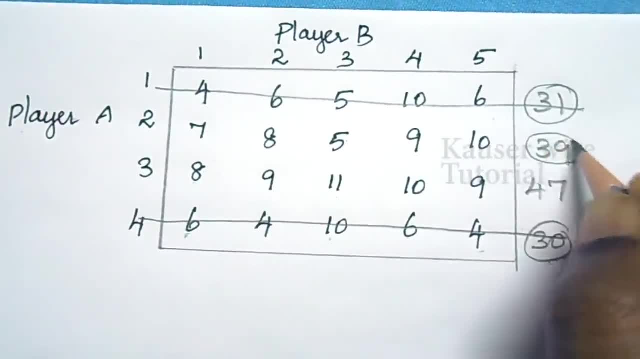 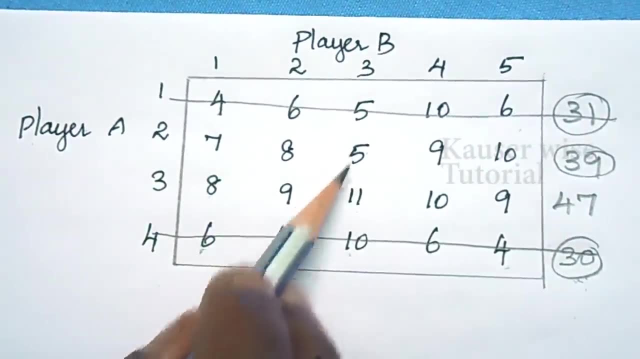 Now let us see the next least value: 39.. So take the 39 and check whether it is dominated by this particular row. 7 is least, 8 also least, 5 is least, 9 is least, But 10 is greater. 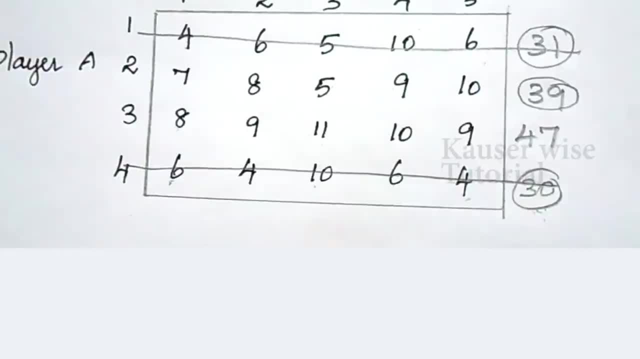 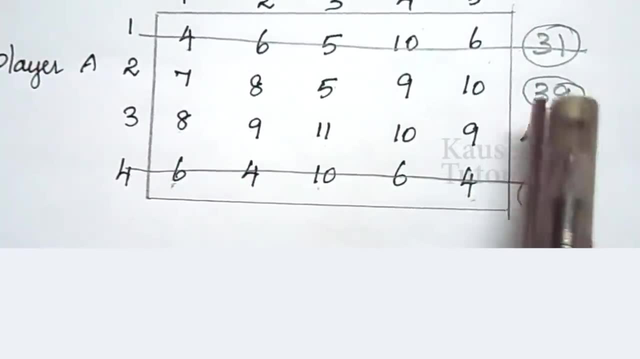 So no continuous domination, See. In pure strategy, we try to reduce the size of the matrix as much as possible. So what is the next value? 47.. So compare these values with the previous one, See. 8 is greater than 7.. 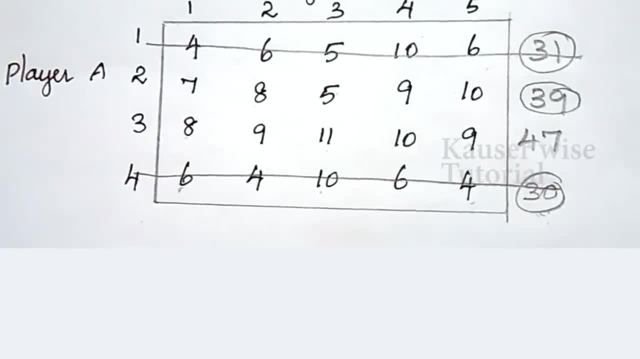 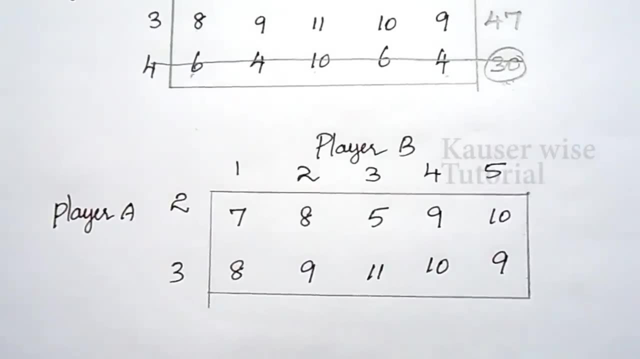 So no dominance. Now we can go for the column reduction After row reduction. now we have 2 rows and 5 columns. Now we need to reduce columns. Okay, For that, first find the total of each and every column. 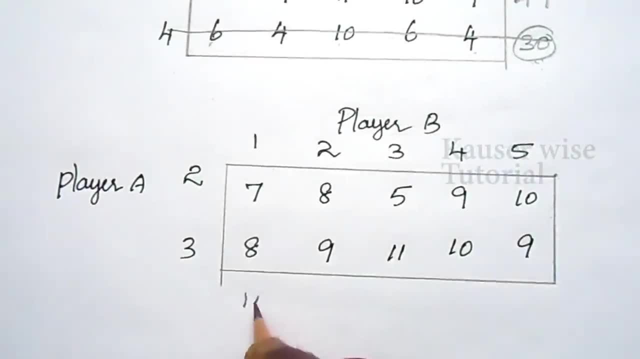 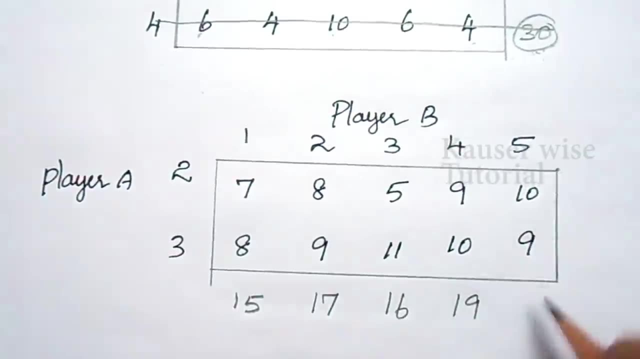 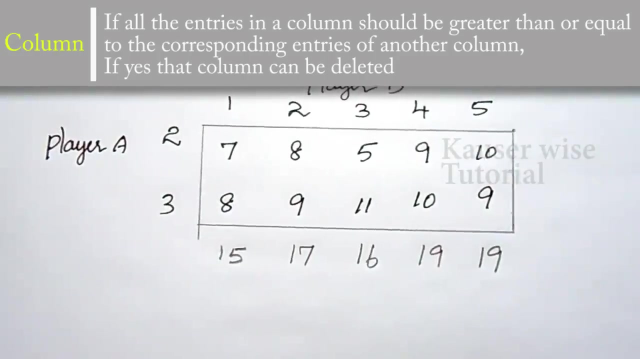 The first column, 7 plus 8. 15.. Second column: total 17.. Third one, 16.. Fourth one, 19. And fifth also 19.. What is the dominance property for column reduction? The selected column element should be greater than or equal to any other column. 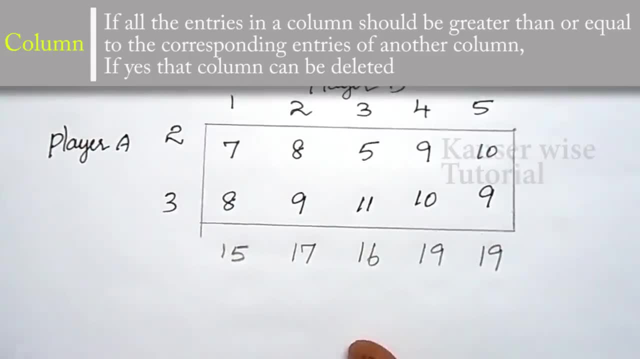 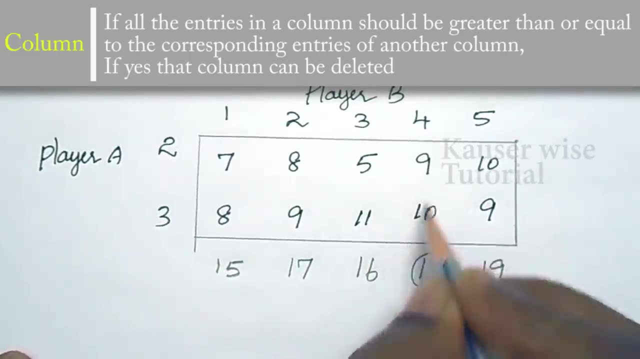 Then the selected column can be deleted. Okay, For that I am going to select the highest value. So here we have got 2 19s. Now take the first one And compare these values with the other elements. So let me start with the first column. 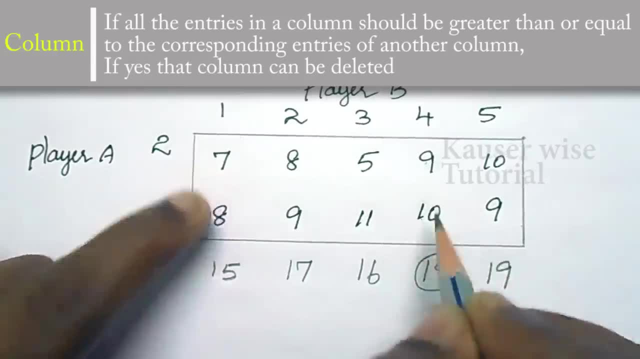 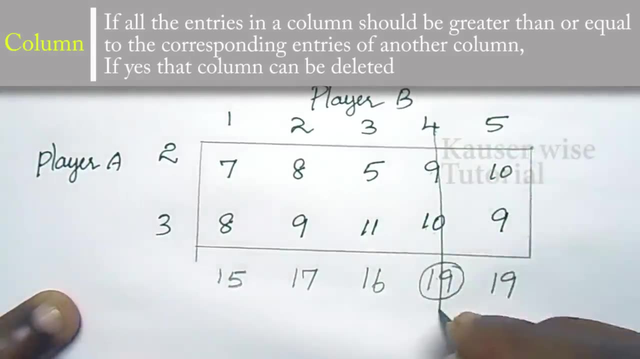 7.. Okay Here, 9.. 9 is greater than 7.. 10 is greater than 8.. This column is dominated by the first column, So delete this. Go to the second highest Again, 19 we have. 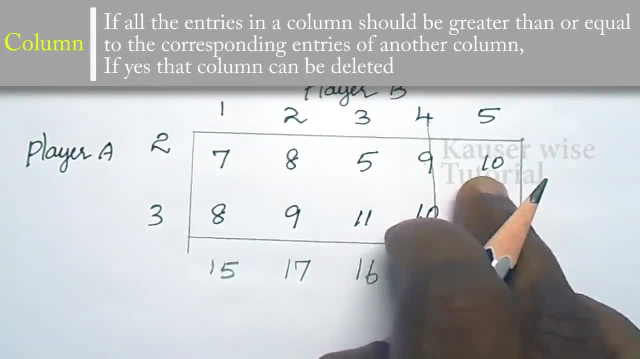 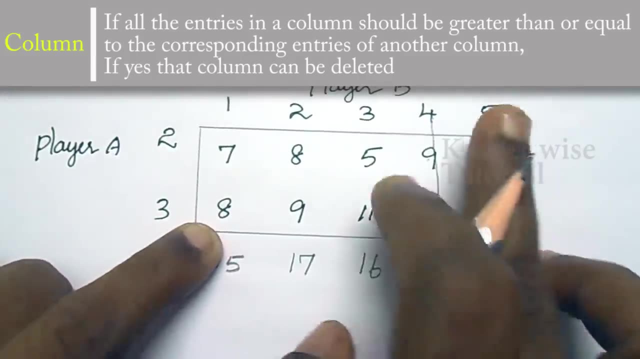 Select this particular column and compare with the other elements. So take the first one: 10 is greater than 7. And again 9 is greater than 8. So this particular column is dominated by first column, So delete this. 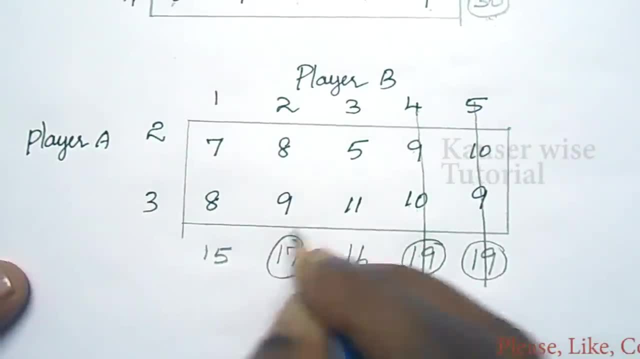 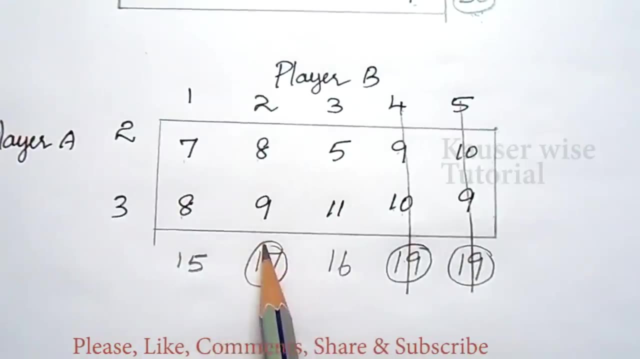 Next highest, 17.. Select this particular column and compare: 8 is greater than 7.. Again, 9 is greater than 8.. So this column also dominated by the first column. So delete this column. Now we have only 2 columns. 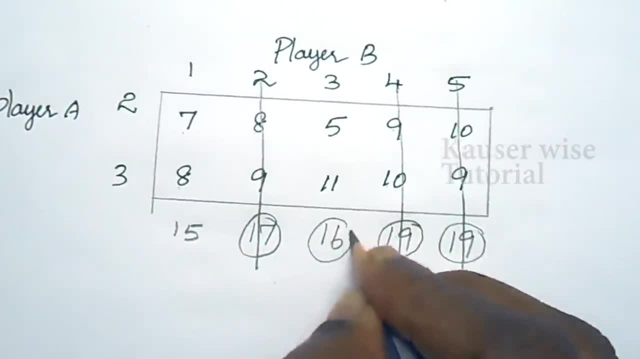 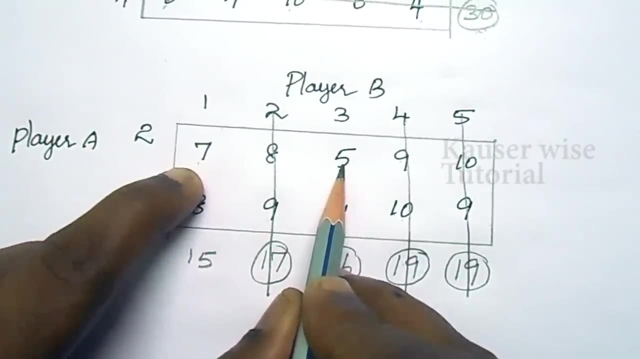 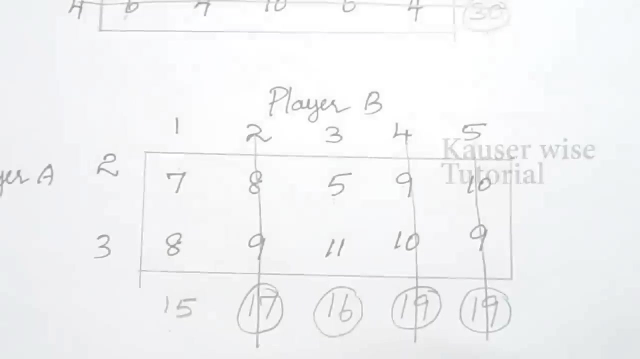 Okay, What is the next highest? 16.. Okay, Select this particular column: See 5, 7.. 5 is lesser than 7. So no domination. See, in pure strategy, we try to reduce the size of the matrix as much as possible. 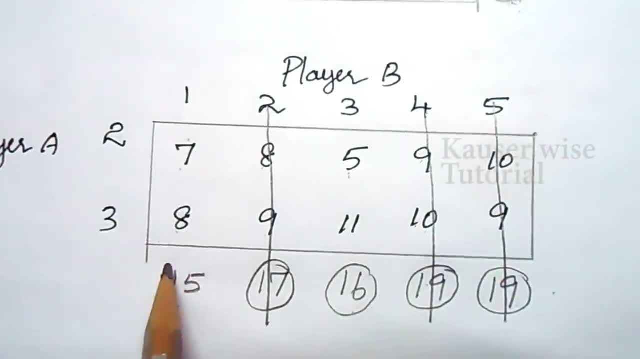 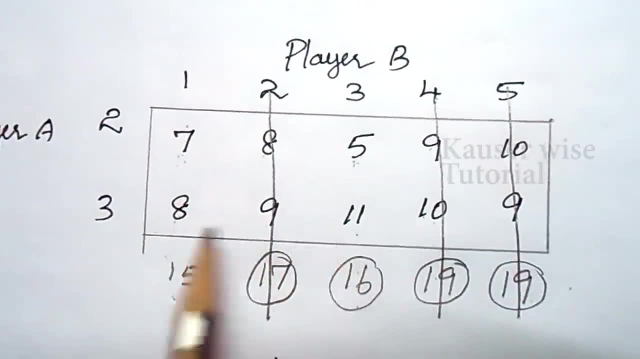 Now go to the last option. Okay, See this particular column and compare with this particular column: 7 is greater than 5.. Okay, And 8 is lesser than 11.. So no continuous dominance. Now we can go for the next option, that is, row reduction. 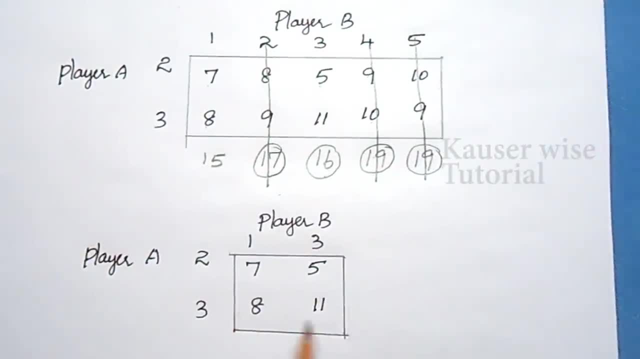 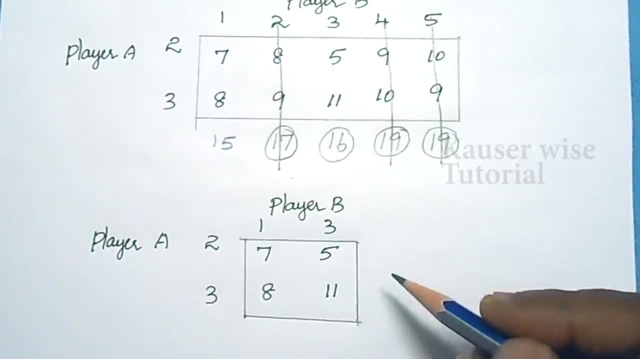 See: after column reduction. Now we have 2 rows and 2 columns. Now we can go for row reduction. We have 2 rows now. Okay, What is the procedure? The selected row value must be lesser than or equal to others. row value. 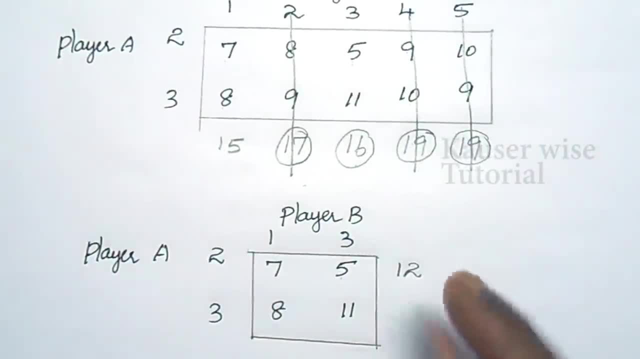 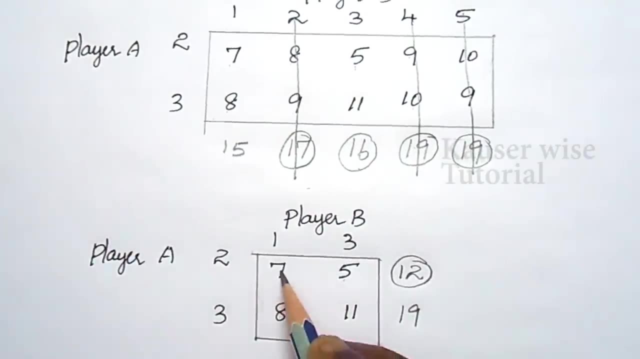 Okay, Look at the first one, 12., And second one, 19.. So which one is least? 12 is least. And compare this value with the other row: 7 is less than 8. And 5 is less than 11.. 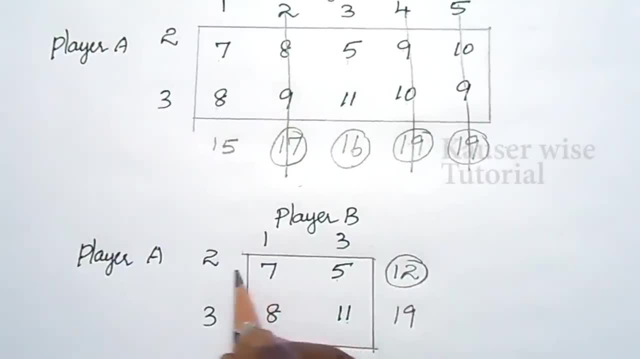 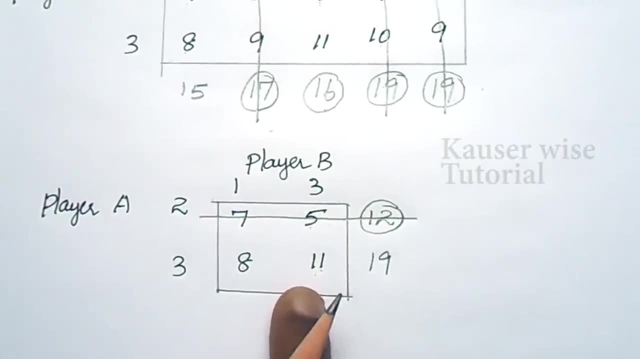 So this particular row is dominated by second row, So delete this row. So now we have only 1 row. Now we can go for column reduction. The selected column must be greater than or equal to other column. Okay, 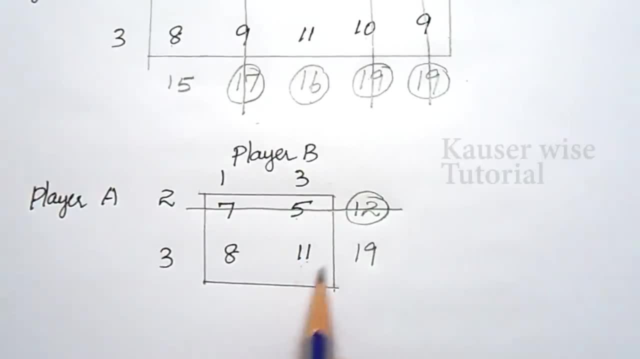 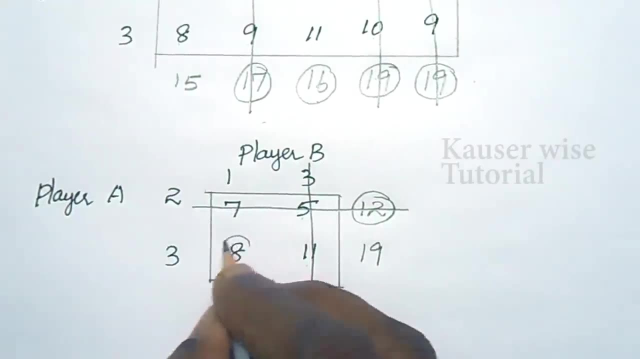 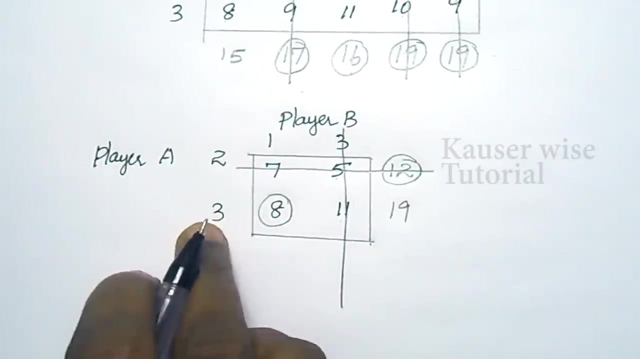 We have 2 columns now, So which one is highest value? 11 is the highest value, So this will be got cancelled, So we have only 1 element. This is the selected strategy. Okay, So player A need to select third strategy. 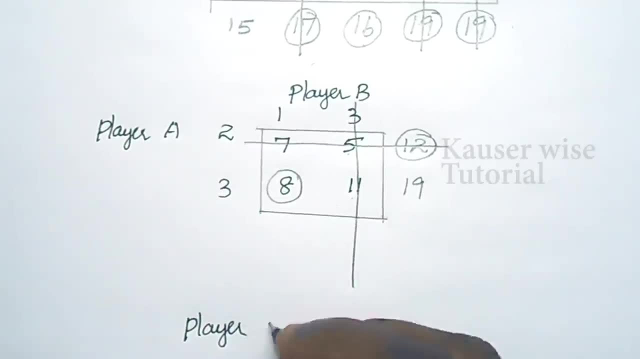 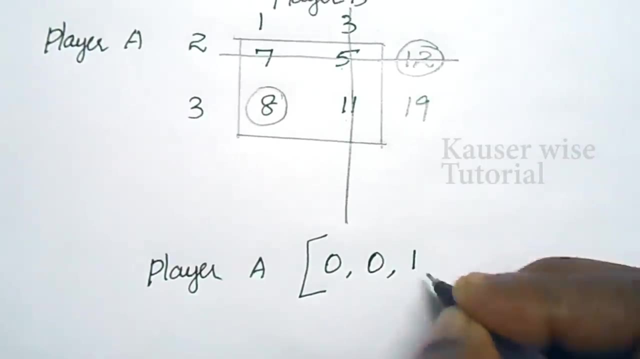 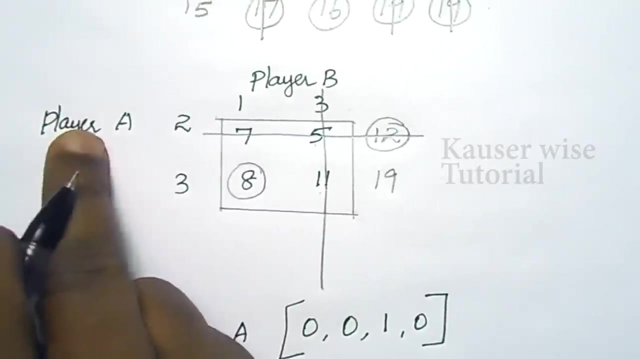 Okay. The remaining strategy probability will be 0.. For player A, probability is first strategy: 0,. second one: 0,. third one selected. fourth one: 0.. Okay For player B. player A need to select third strategy and player B need to select the first. 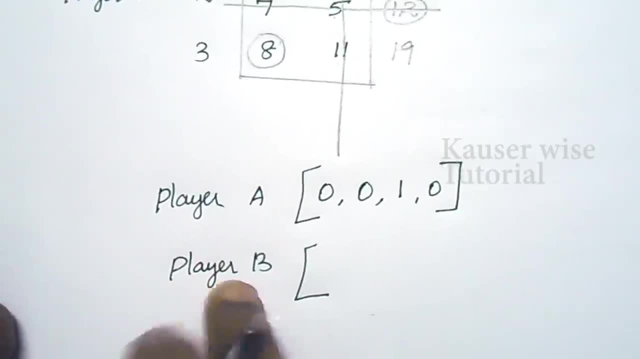 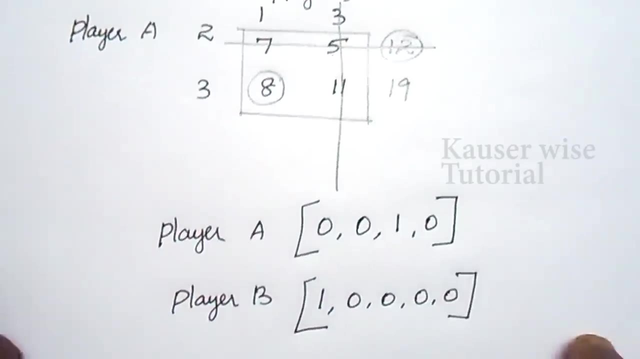 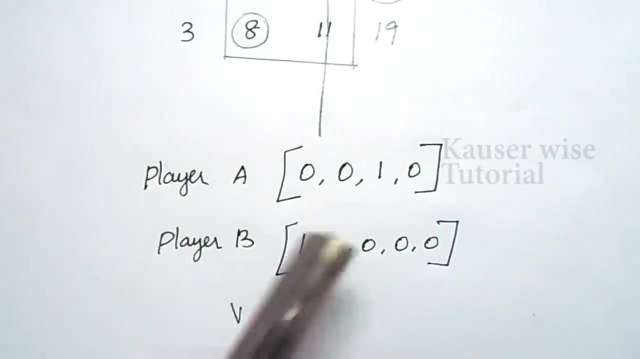 strategy. The probability is for player B. he is going to select the first strategy. The remaining strategy probability will be 0.. Okay, The value of the game is 8.. This is the way to find the value of the game and probabilities of player A and player B. 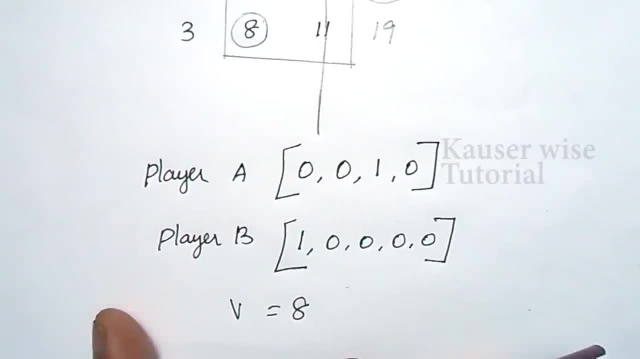 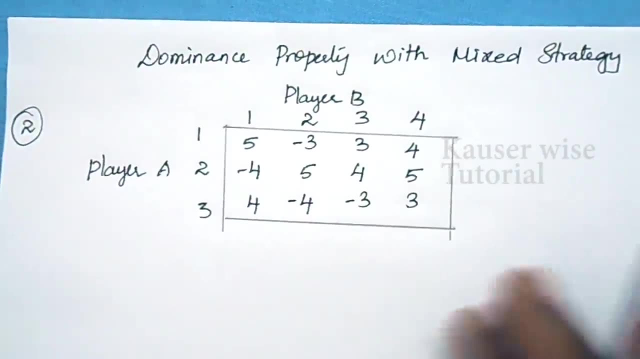 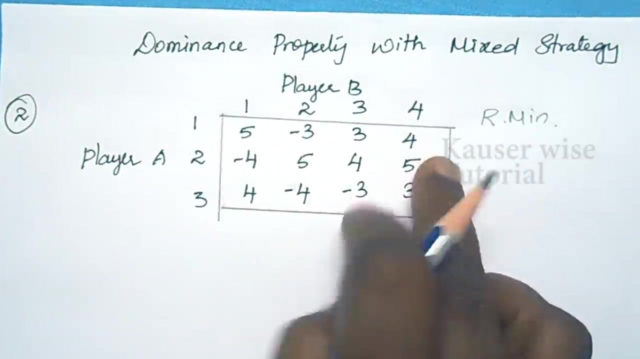 by using dominance property with pure strategy. Look at the second problem. Now. I am going to solve this problem by using dominance property with mixer strategy. Okay, First we need to find the row minimum. In the first row, minimum value is minus 3.. 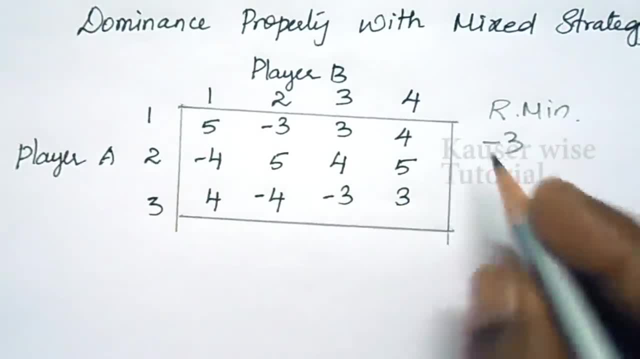 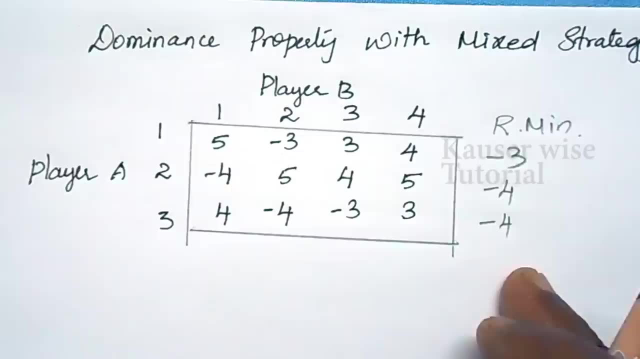 In the second row, minimum value is minus 4.. In the third row, minimum value is minus 4.. Among these minimum value, which one is maximum value? Minus 3 is the maximum value. Now find out column maximum. 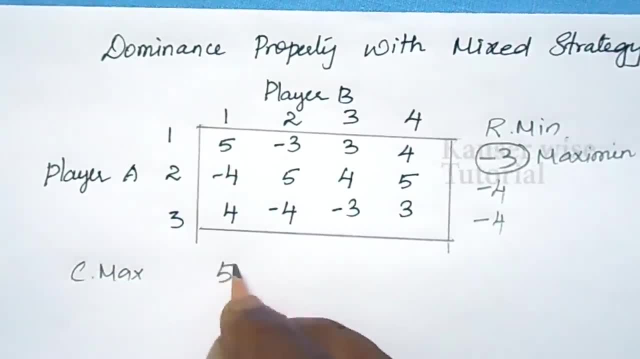 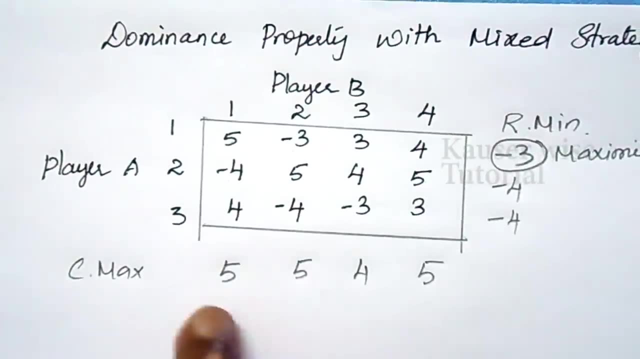 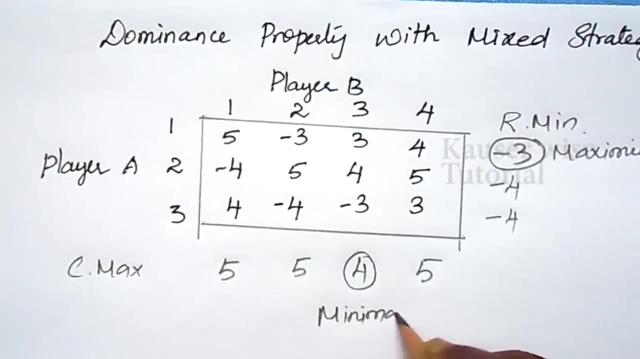 In the first column, maximum value is 5.. Second column: also 5.. Third column: 4.. Fourth column: also 5.. Okay, Among these values, which one is minimum value? 4 is the minimax value. Okay, Now, this point has no saddle point. 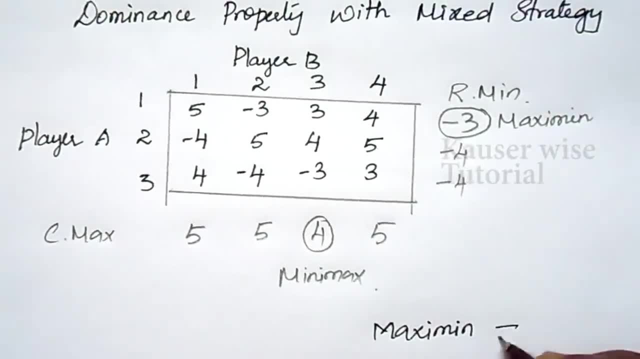 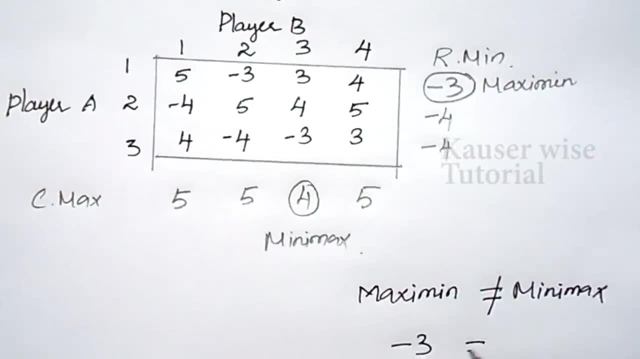 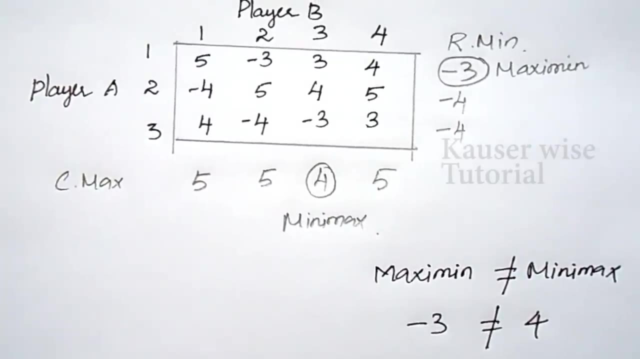 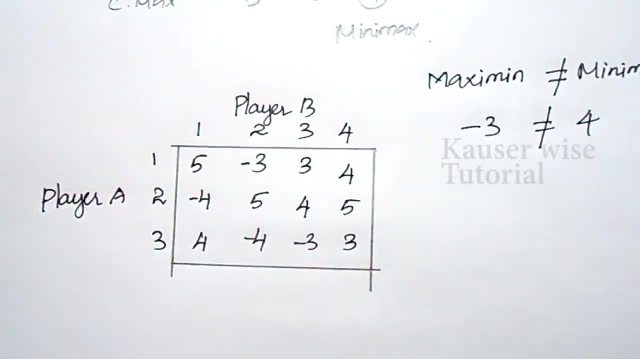 Why? Because maximum value is not equal to minimax value. Okay, Maximum value is minus 3 and minimax value is 4, which is not equal. Now you need to proceed. dominance property to reduce row and column. Okay, In order to eliminate the row, just find the total of each and every row and find out the least one. 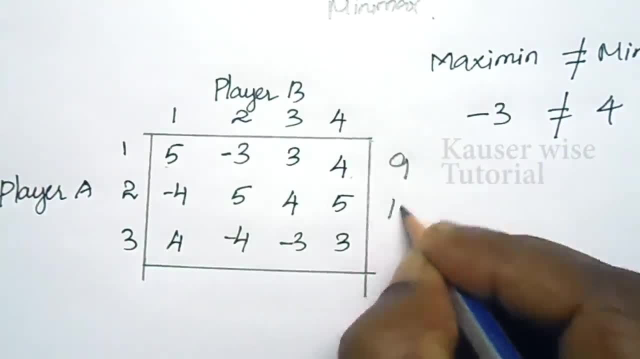 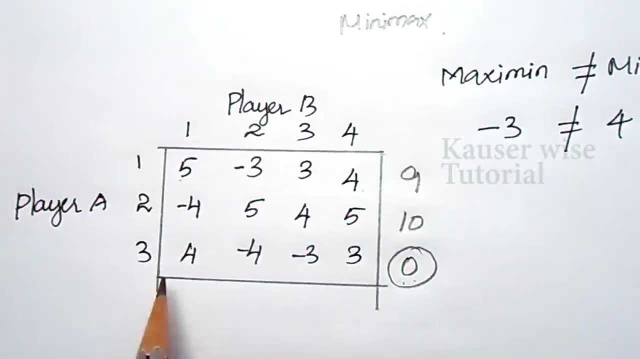 First row total is 9.. Second one, 10. And the third one, 0.. Among these values, which one is least? 0 is the least value. So just check these rows values, whether these values dominated by any other row. 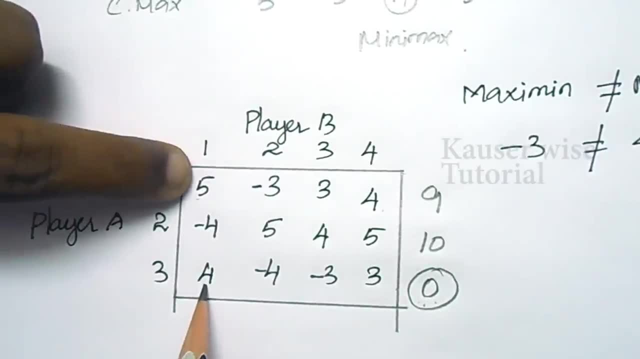 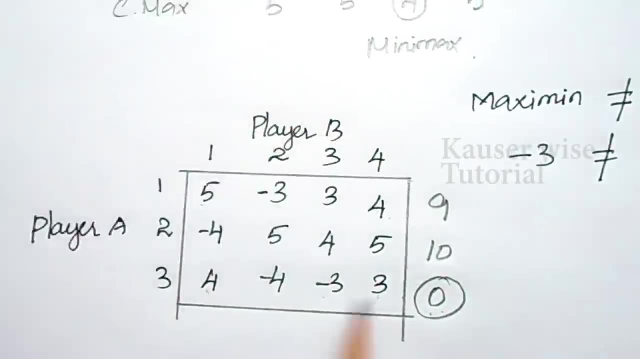 I am going to start with the first row. Okay, 4 is lesser than 5.. Minus 4 is lesser than minus 3.. Minus 3 is lesser than 3.. And 3 is lesser than 4.. So this particular row is dominated by first row. 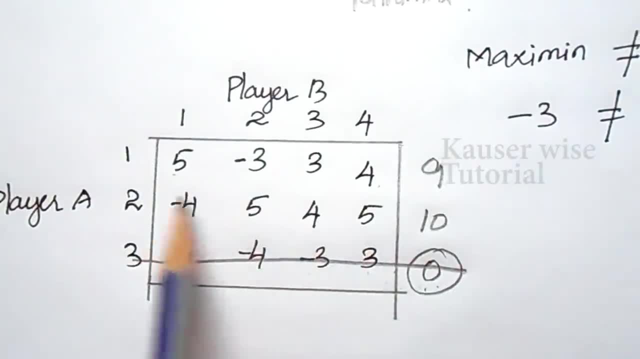 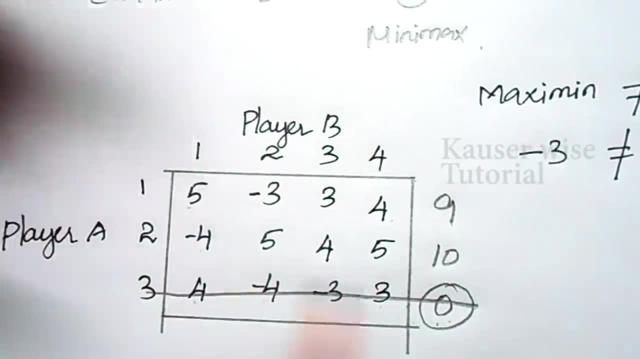 So delete this row. Now we have only 2 rows. The next least value is 9.. Now just check this particular row. Okay, 5 is greater than minus 4.. So no dominance. The next value is 10.. 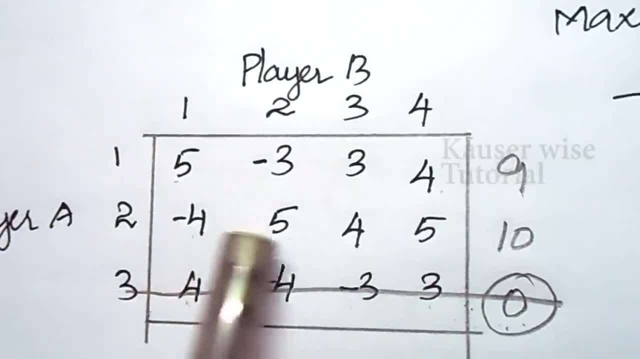 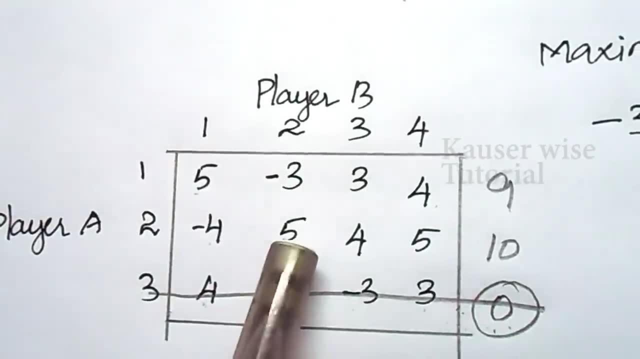 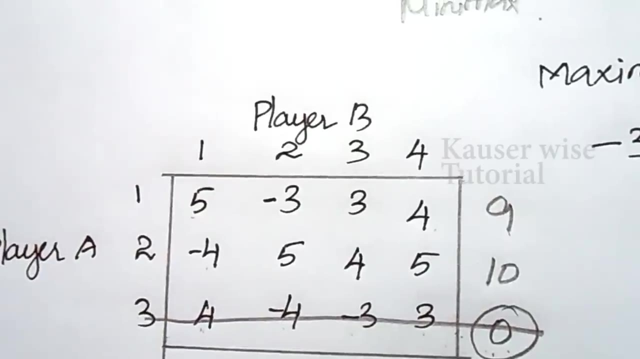 Okay, This is the last possibility. Now compare these values with the previous row. Minus 4 is lesser than 5.. 5 is greater than minus 3.. So no dominance. So now we can go for column reduction in order to reduce the payoff matrix into 2 by 2.. 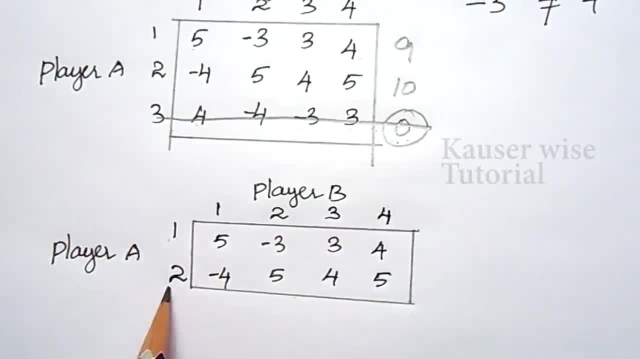 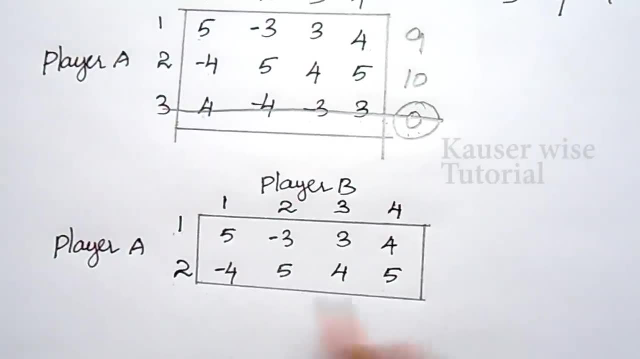 After the elimination of third row. now we have first row and second row and 4 columns. Now we need to reduce the column Now. for that, just find the total of each and every column. The first column total is 1.. 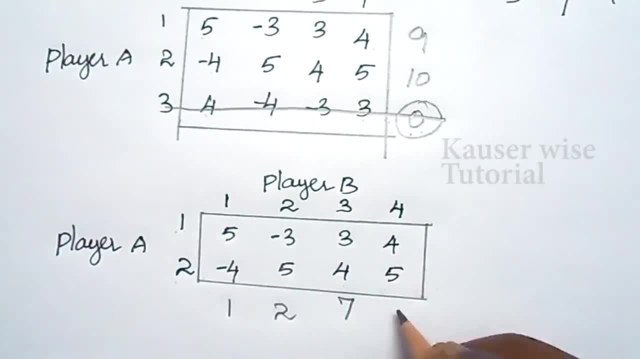 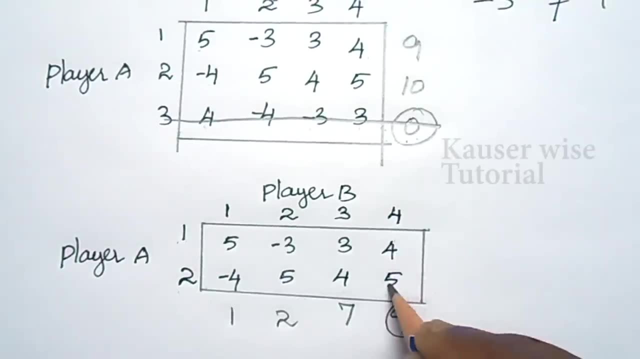 Second one, 2., Third one, 7. And fourth one, 9.. So, among these values, which one is highest value? 9 is highest value. Now compare these values with the other column in order to eliminate this particular column. 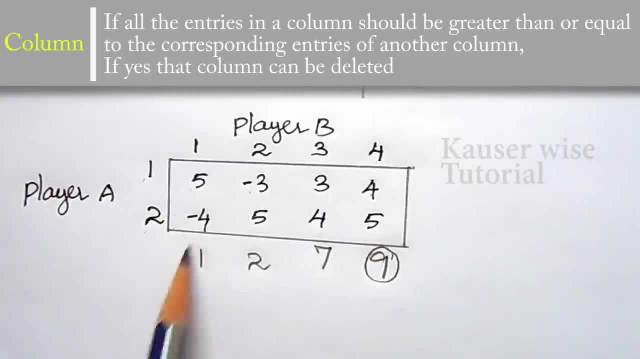 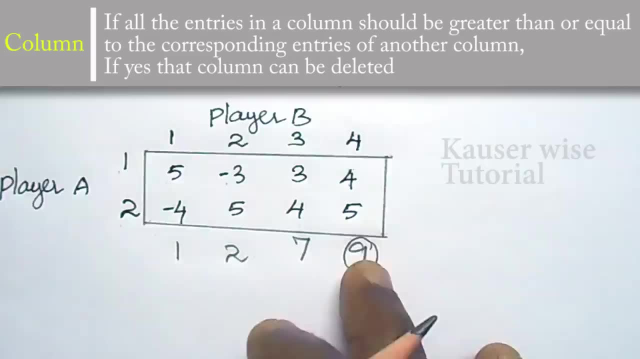 So now I am going to compare these values with the other column to check the dominance property rule. Okay, The dominance property rule for column S: the selected column value must be greater than or equal to other columns. Okay, Now I am going to start with the first column. 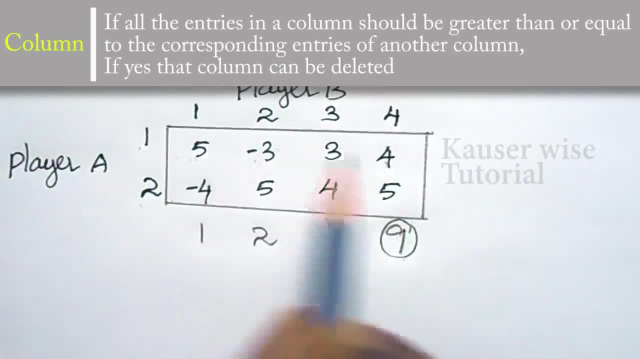 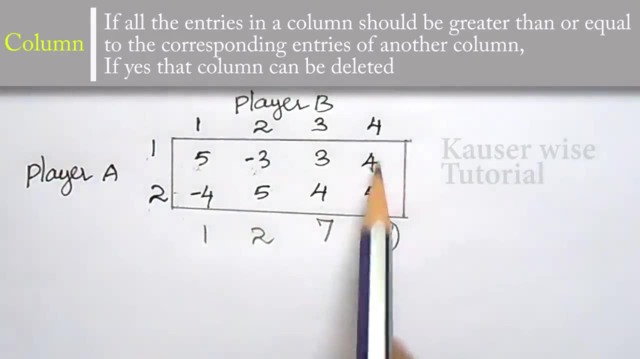 The first column value is 5.. This one is lesser value, So no dominance. Go to the second column Minus 3, 4.. 4 is greater, 5, 5 equal. So this particular column is dominated by second column. 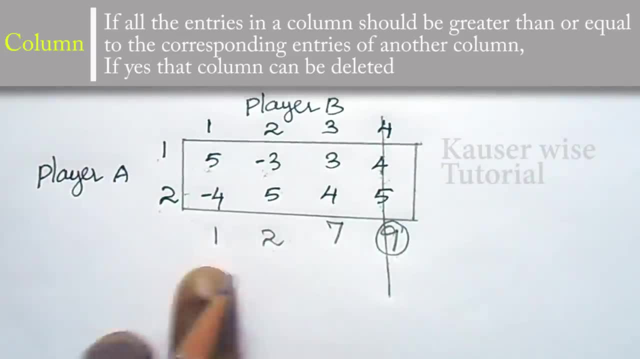 So this one will get cancelled Now. next highest value is 7.. So now I am going to compare this column values with the other column values, So let me start from the first one. Okay, 5, 3.. 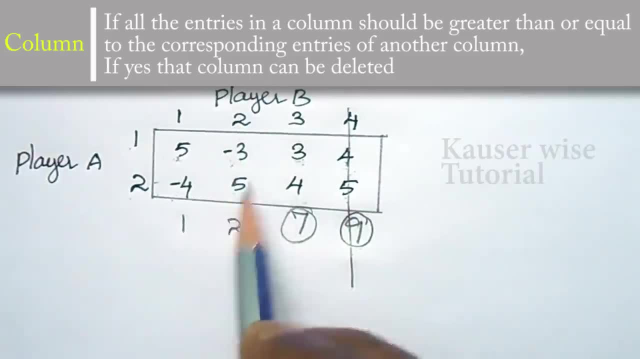 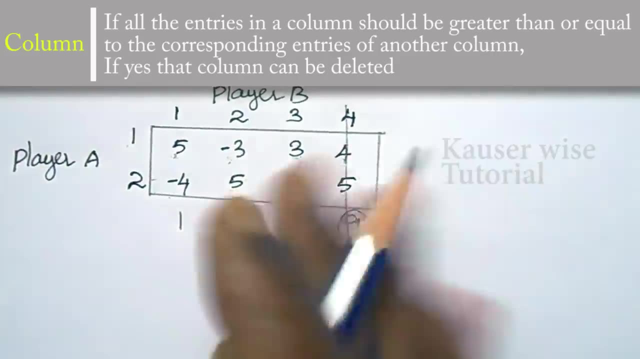 Okay, 3 is least value, So no dominance. Go for the second one, Minus 3, 3. Yes, Higher value: 5, 4. Least, So no dominance. Okay, Now you can go to the other option. 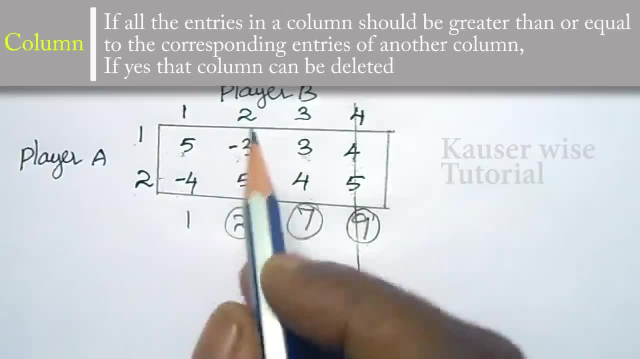 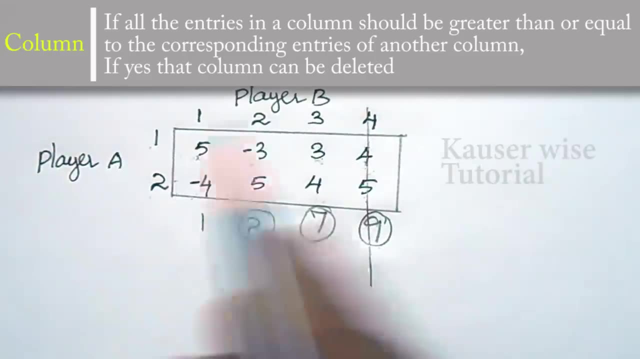 Now I am going to select this column. Okay, Let me check the dominance property: Minus 3,- 5.. Least value: No dominance. Minus 3, plus 3. No dominance. Let me see the last option. 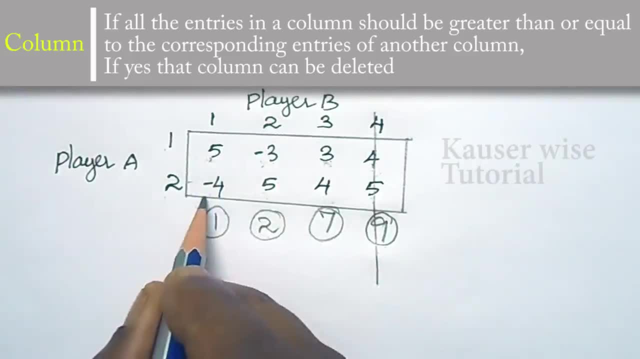 5, minus 3.. Yes, Greater value, Then minus 4, 5.. No dominance. Go to the last option: 5, 3.. Yes, Higher value, Then minus 4, plus 4.. 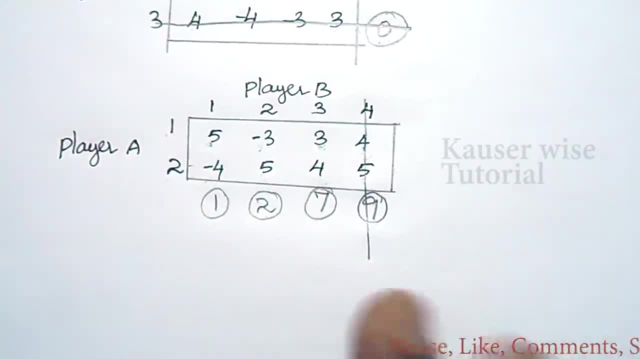 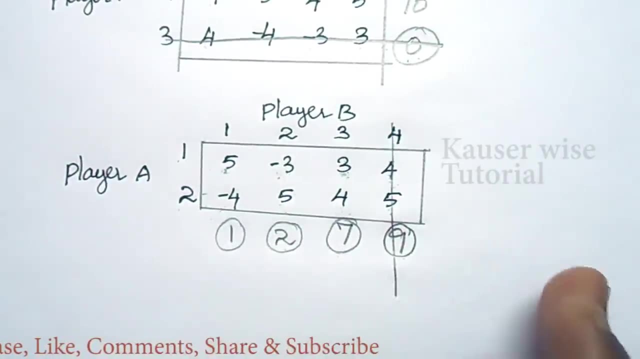 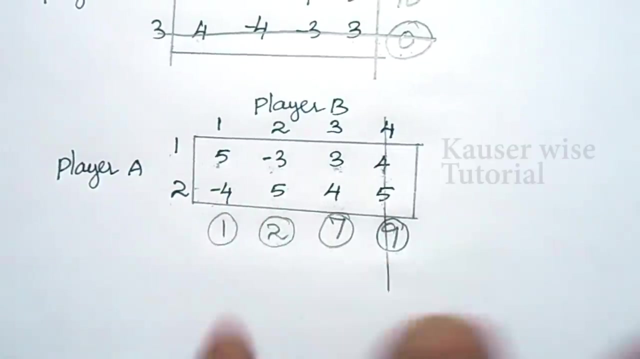 No dominance. So now, in this situation, you can take average of any two columns and compare with the other column in order to check the dominance property. Okay, So now I am going to take the first column and second column average, So 5, minus 3, divided by 2.. 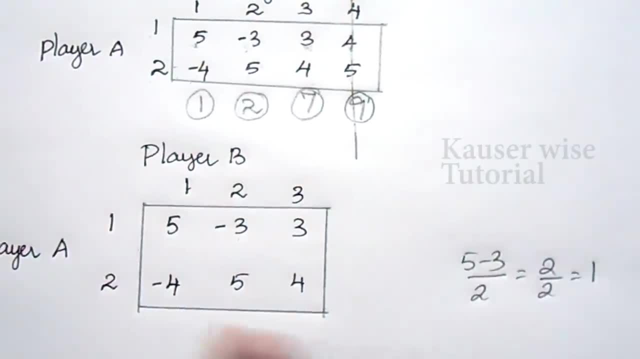 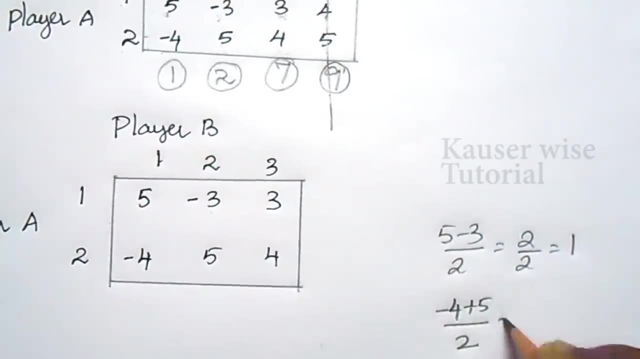 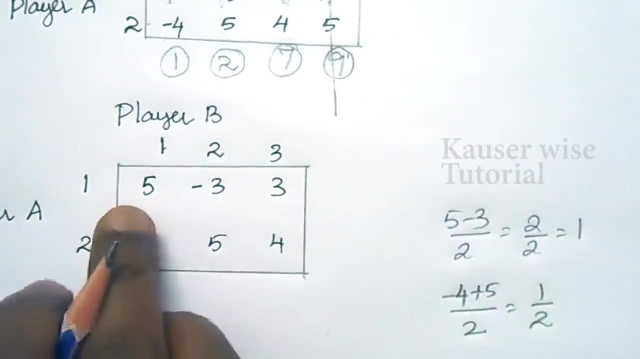 2 by 2 is equal to 1.. Minus 4, plus 5, divided by 2.. 1 by 2.. Okay, Now I am going to compare these values with the third column. This is the average of 1 and 2, and this is the average of minus 4 and 5.. 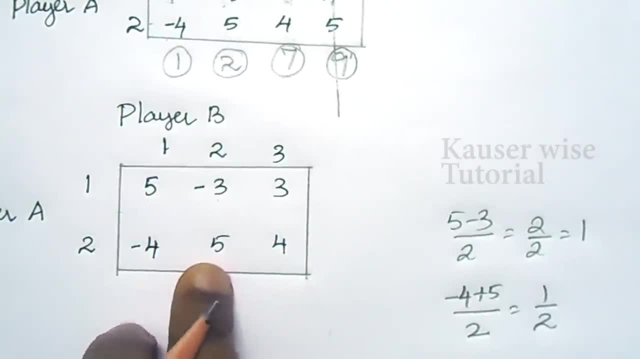 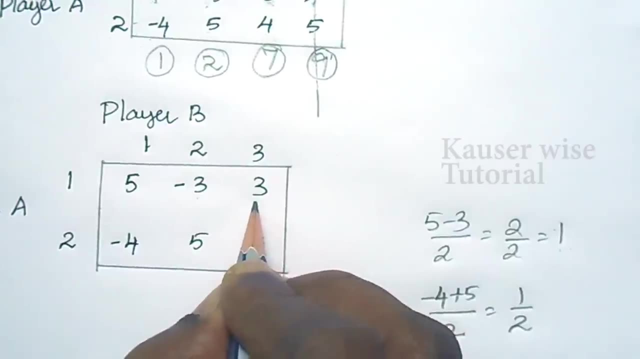 Now compare the average value with the third column. Okay, The first one is 1 and this one is 3.. 3 is higher value. Next, 1 by 2 is 4.. 4 is higher value. This particular column dominates the average of one column. 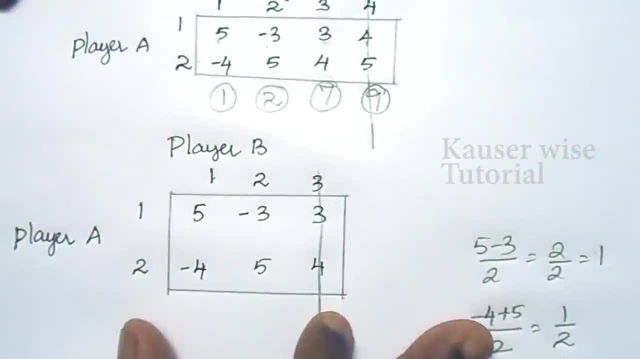 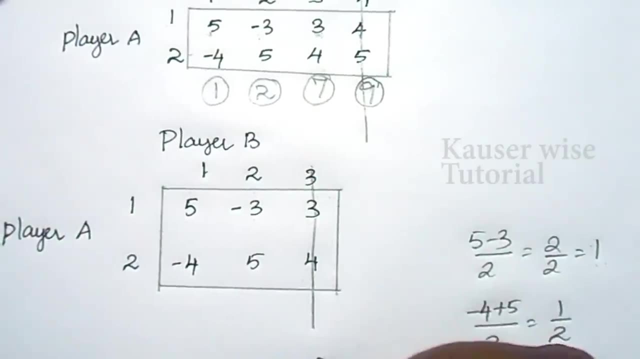 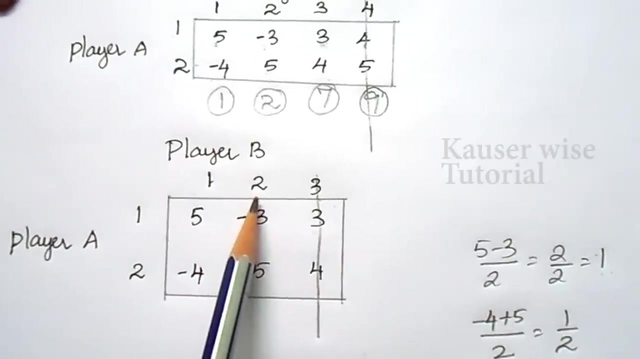 average of 1 and 2, so got cancelled here. i have taken average of first and second column and compare with 3. okay, if you could not eliminate any one particular column, you can go for other option. the other options are: you can take average of 1 and 3 and compare with 2, or you can take 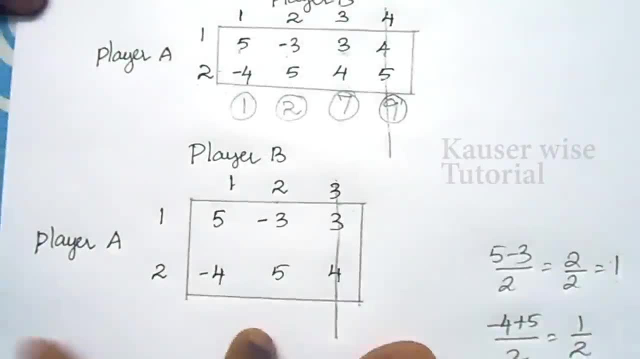 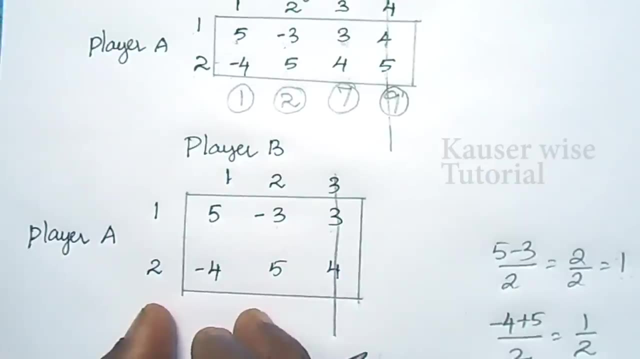 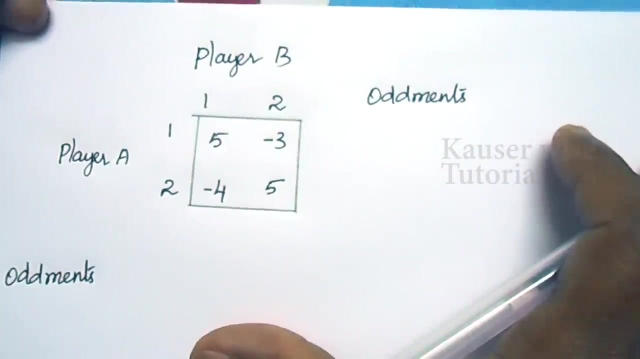 average of 2 and 3 and compare with 1. but here the third column got cancelled. now we have got 2 by 2 payoff matrix. with this we can proceed to find out the probabilities and value of the game. okay, in order to find out the probabilities and value of the game, first you need to find out the 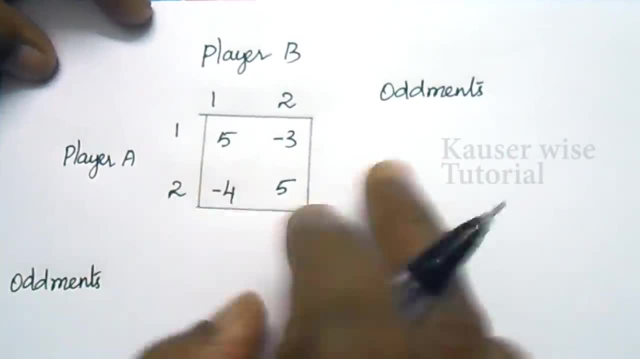 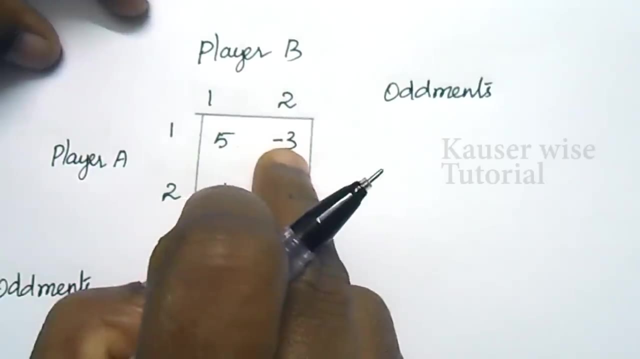 oddments, row oddments and column oddments. so the first one. find the difference between these two and write it again. so, second row: okay, 5 minus minus 3 is equal to 8. in the same way, for the second row, 5 minus 3 is equal to 8. in the same way, for the second row, 5 minus 3 is equal to 8. 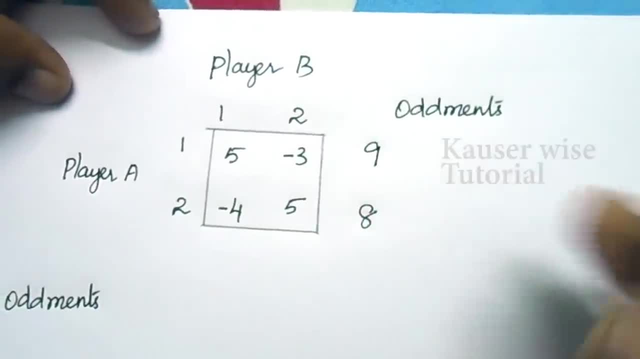 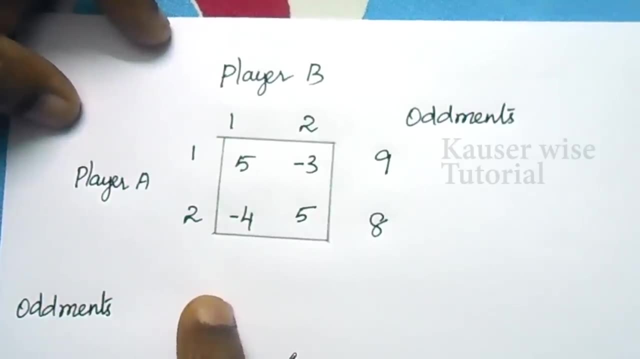 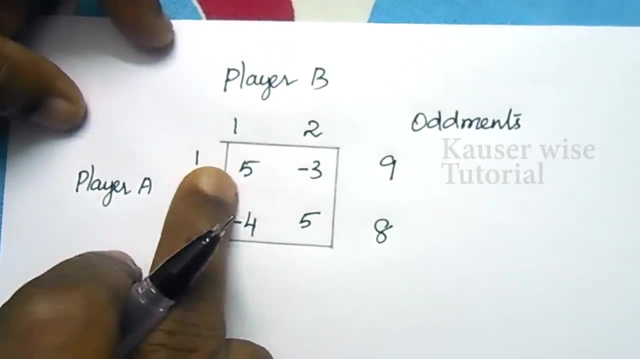 minus minus 4 is equal to 9. in the same way, you need to find the oddments for first column and second column. and find the oddments for the first column and write it against second column, and find the oddments for second column and write it against first column. so 5 minus minus 4 is equal to 9. 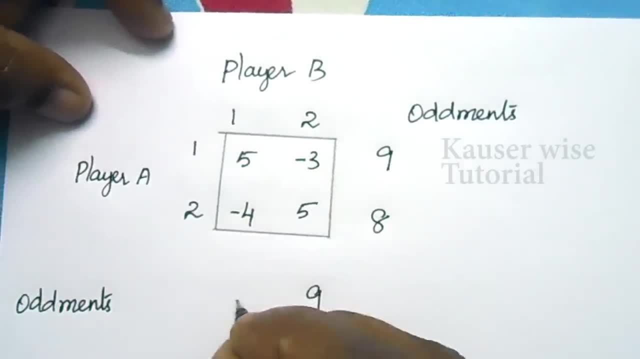 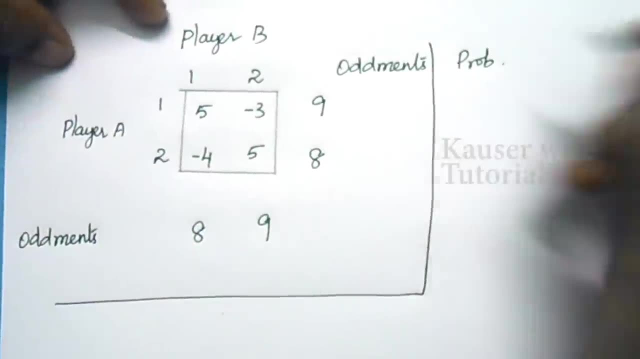 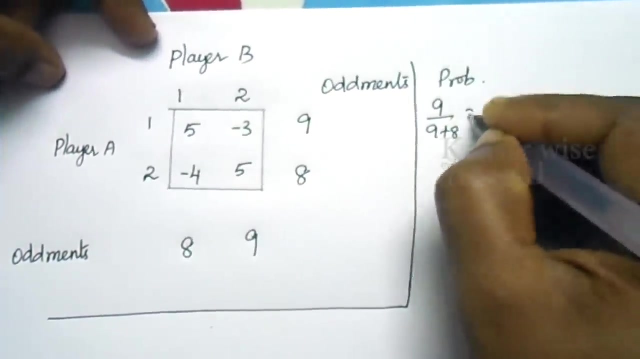 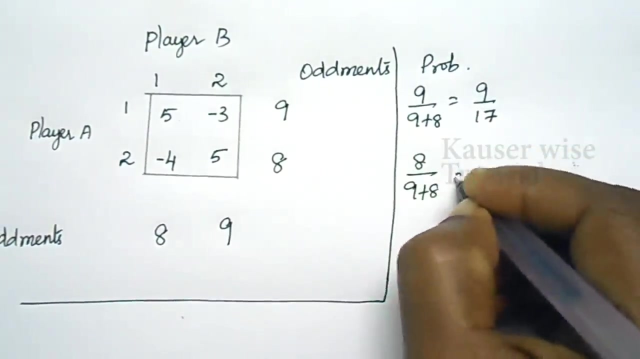 and 5 minus minus 3 is equal to 8. these are the row oddments and column oddments. now we can go for the probabilities. okay, for the first one, 9 divided by 9 plus 8 is equal to 9 by 17. for the second row, 8 divided by 9 plus 8 is equal to 8 by 17. in the same way, 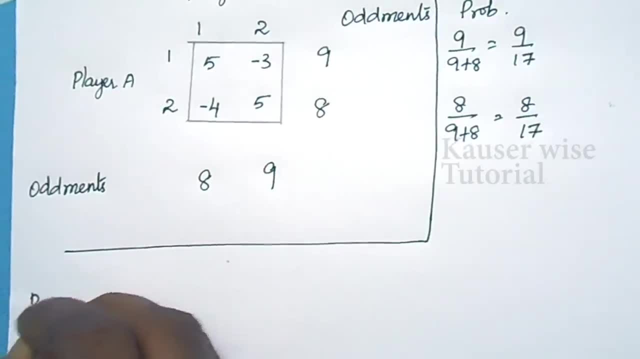 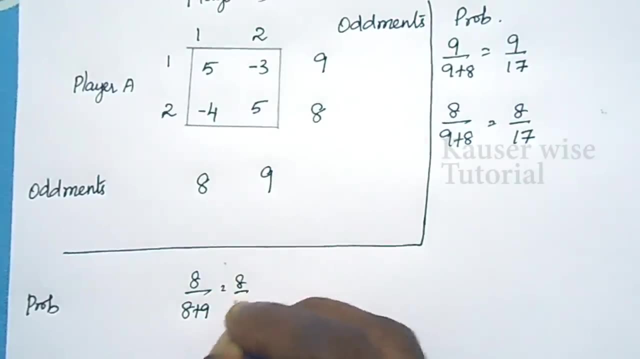 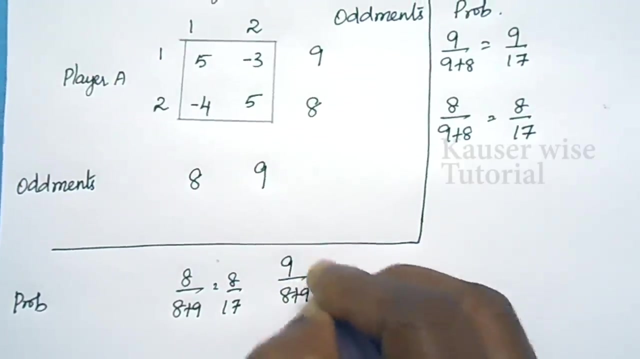 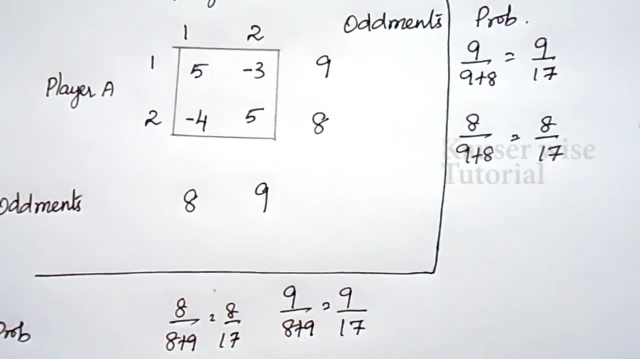 find out the probability for columns also: 8 divided by 8 plus 9 is equal to 8 by 17. for the second column, 9 divided by 8 plus 9 is equal to 9 by 17. these are the probabilities of row and column. now you can find the value of the game. so what is the procedure? 5 into 9 plus minus.